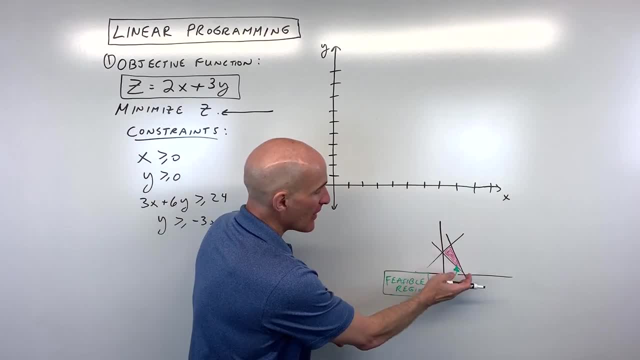 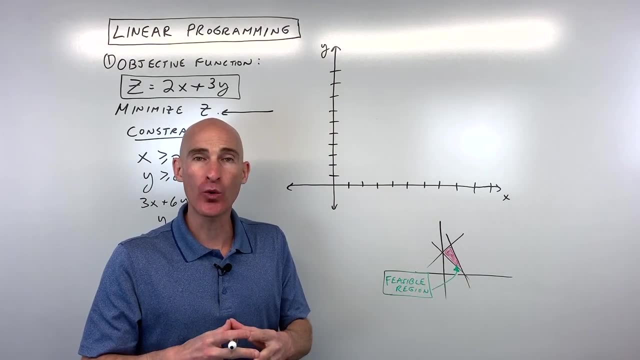 So just a bird's eye view. what you're trying to do is you're trying to graph these linear inequalities and what you get is an overlapping region that satisfies all those constraints, or those inequalities, And this red region here. I'm just showing you an example. 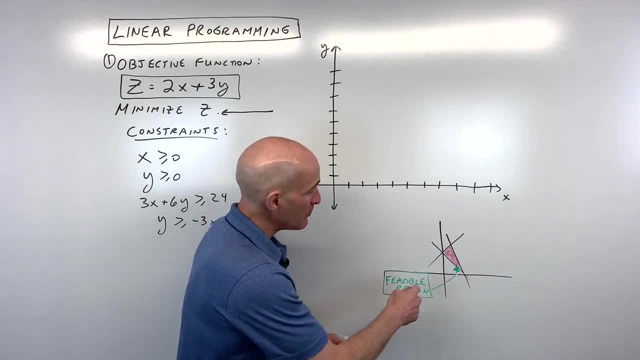 this would represent what's called our feasible region, and if you pick any point in that region, it satisfies the constraints. But what's interesting is that at the vertices, at these points, on this polygon that's formed here will give you either a maximum value or a minimum. 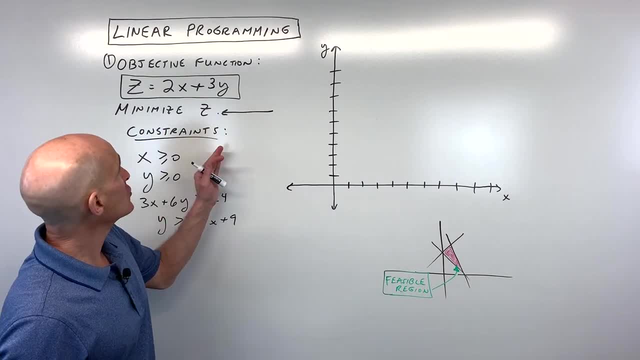 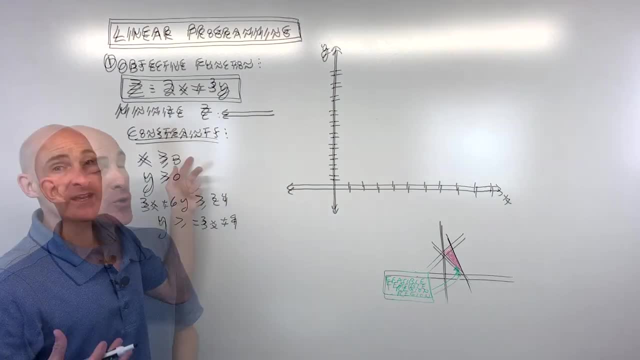 value, depending on what you're trying to find. So let's go ahead and do a basic example first, where we're trying to minimize, and then we're going to do a word problem where we're going to try to maximize. Okay, so for number one, our objective function is this: z equals 2x plus 3y. 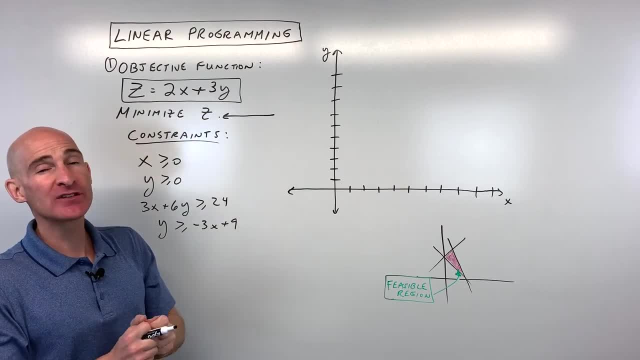 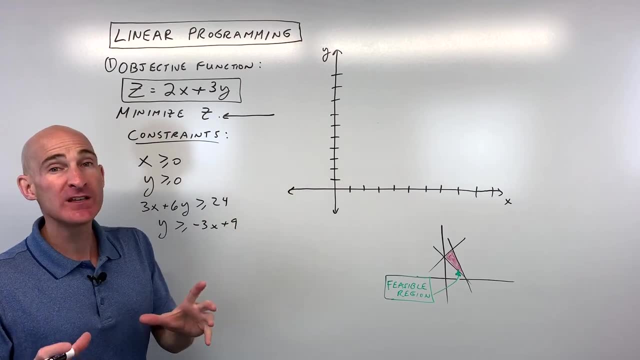 What we want to do is we want to minimize z. we want to find the smallest value for z. Now the constraints, these are our restrictions or these are our inequalities. we want to graph to get our feasible region. So x is greater than or equal to zero. that's a vertical line. 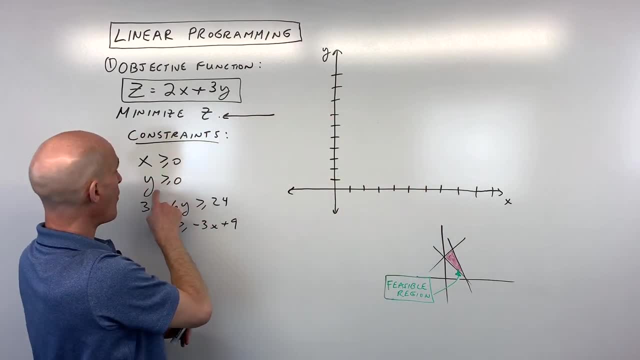 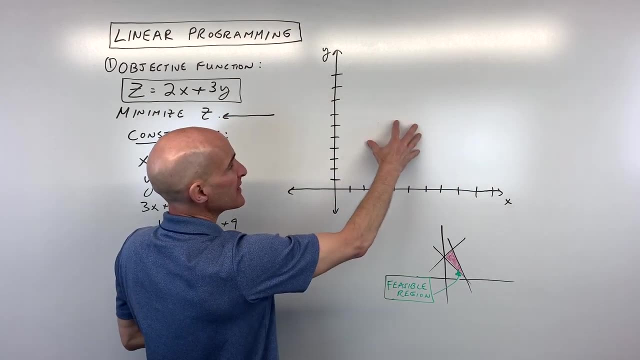 and greater than we're going to be shading to the right. y is greater than or equal to zero. y equals lines are horizontal lines and that's going to be greater than that's going to be above. So what that does is that puts us in the first quadrant. We've got two. 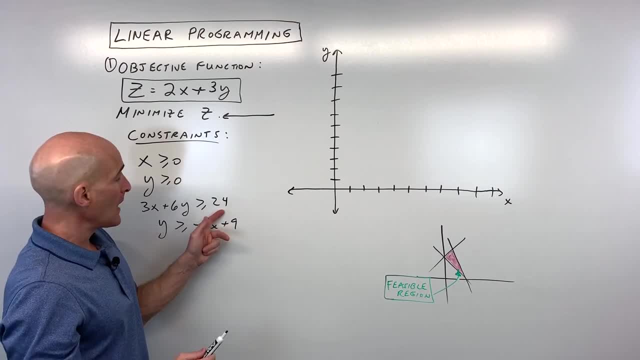 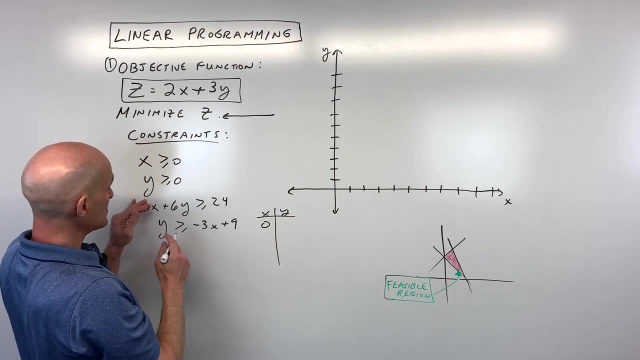 more. we've got 3x plus 6y is greater than or equal to 24.. What I'm going to do for this one is I'm just going to make a table and find the x and y intercepts. So if x is 0,, 3 times 0 is 0,. 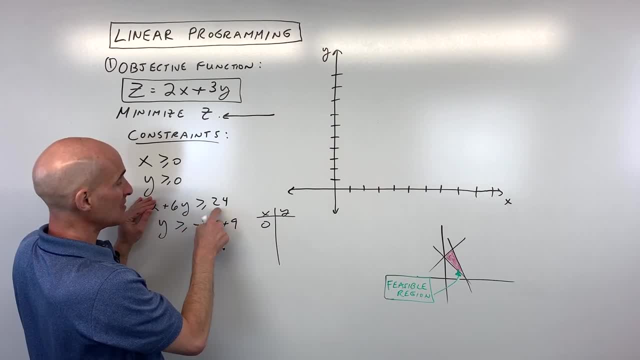 so I'm just going to cover that up. divide both sides by 6 so you can see that y is going to equal 4, and then if I set y to 0,, 0 times 6 is 0, and if I divide by 3 to both sides, x is going to equal. 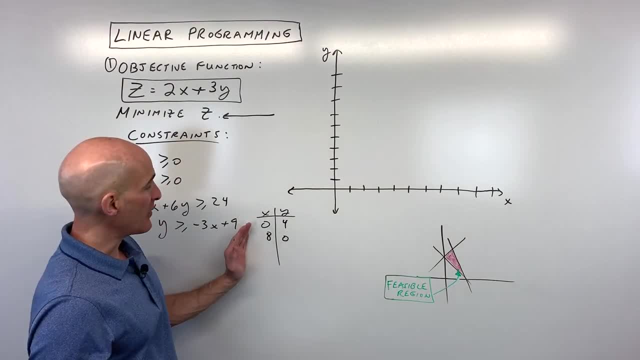 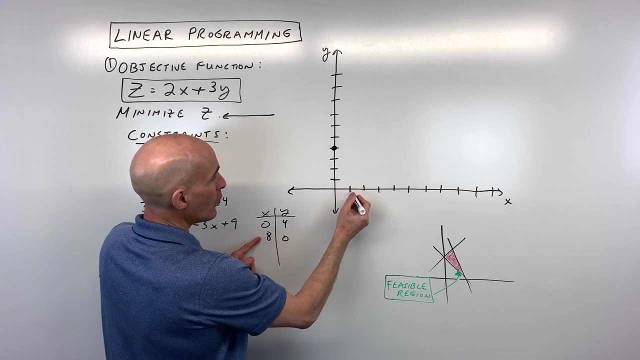 8.. So that's just a quick way. this is called the intercept method of graphing inequality. So we've got 0,, 4, 1,, 2,, 3, 4, that's going to put us right here- and 8, 0,, 1,, 2,, 3, 4, 5, 6, 7, 8, 0.. 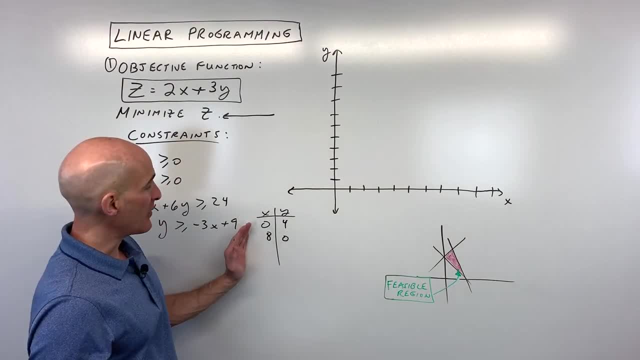 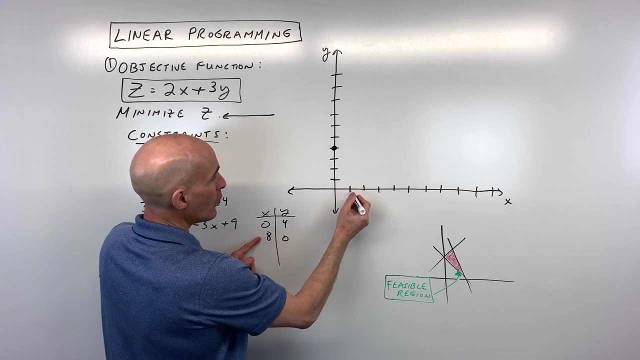 8.. So that's just a quick way. this is called the intercept method of graphing inequality. So we've got 0,, 4, 1,, 2,, 3, 4, that's going to put us right here- and 8, 0,, 1,, 2,, 3, 4, 5, 6, 7, 8, 0.. 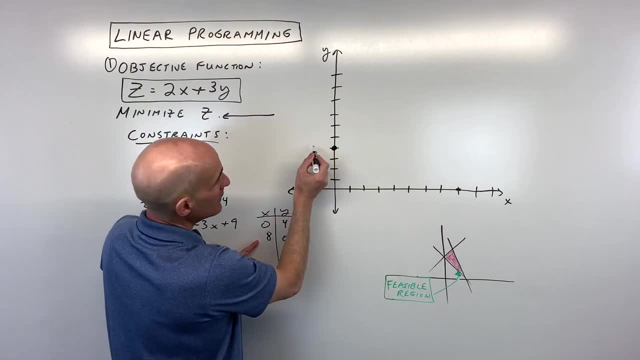 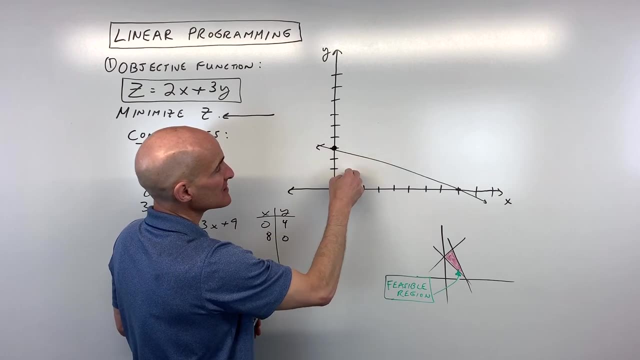 And I'm just going to draw a solid line because it's equal to. and then when you graph using the x and y intercepts like this, you want to pick a point on either side of this line and test it to see if it makes it true. So, for example, if I put 0, 0 in 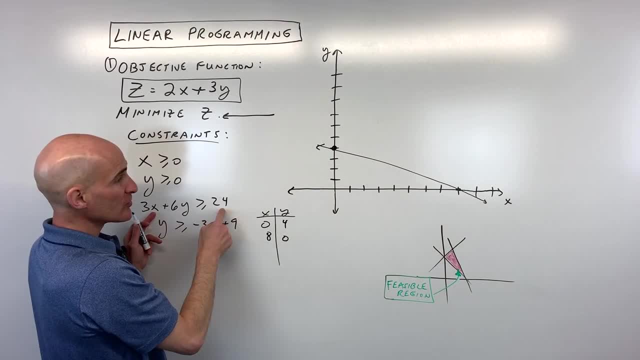 that's the origin. this test point here is 0 greater than or equal to 24? Well, no, So that's means we wouldn't want to shade on this side of the line. we want to shade on this side of the. 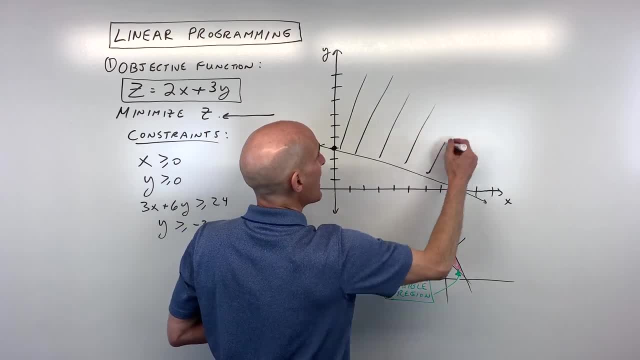 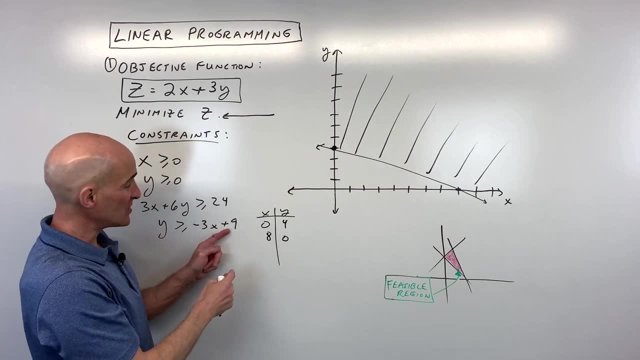 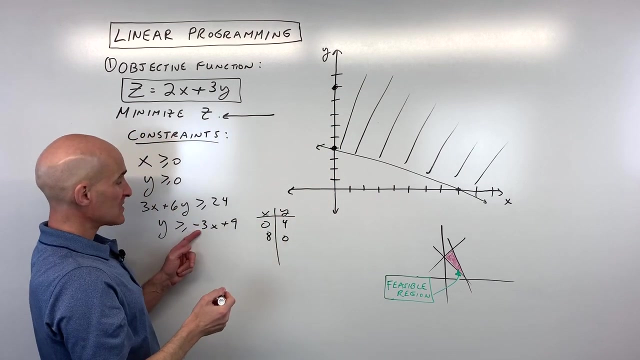 line. So let me go ahead and just draw some lines, just so we know that we're on this side. Okay, for the second inequality, y is greater than or equal to negative 3x plus 9.. So we see that the y intercept is 9, so that's going to be 1,, 2,, 3,, 4,, 5,, 6,, 7,, 8,, 9.. The slope is negative: 3,. 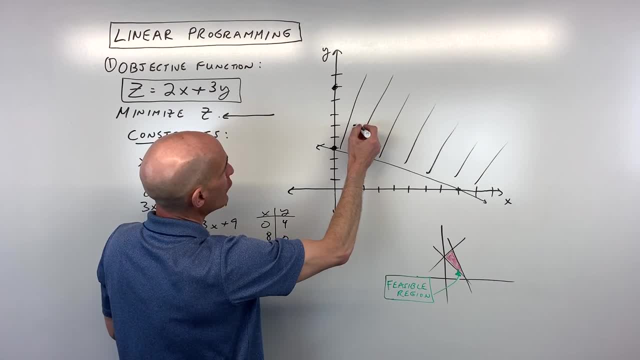 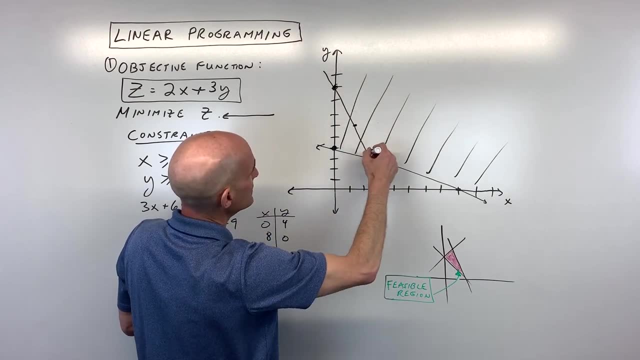 which is like negative 3 over 1, so we're going to go down 3 over 1,, down 3 over 1, so let me just kind of draw this in. Okay, something like that. And this one y is by: 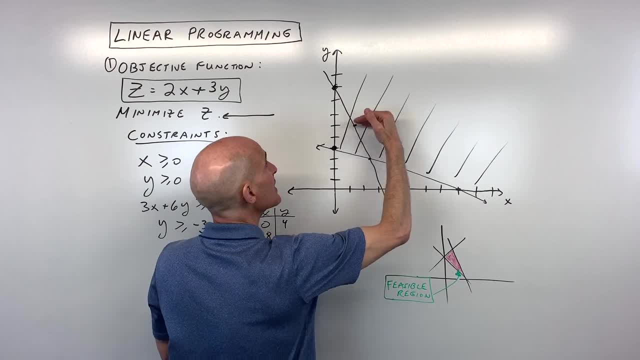 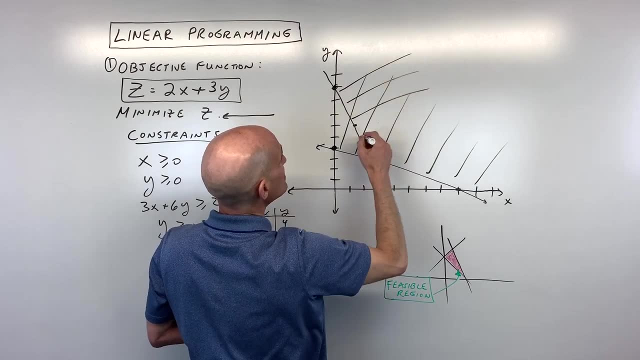 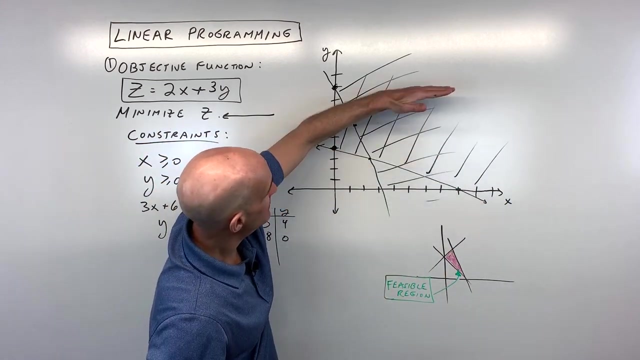 itself and when y is greater than that means that we're going to be shading above the line. So what that means is I'm going to be shading on this side of the line. So let me just draw some lines just to illustrate some shading here. Okay, like that. Now you can see that we were above the 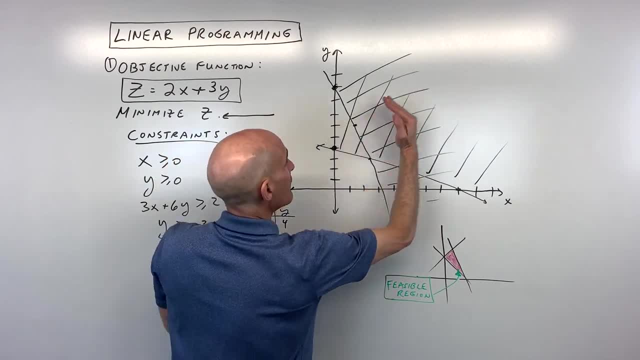 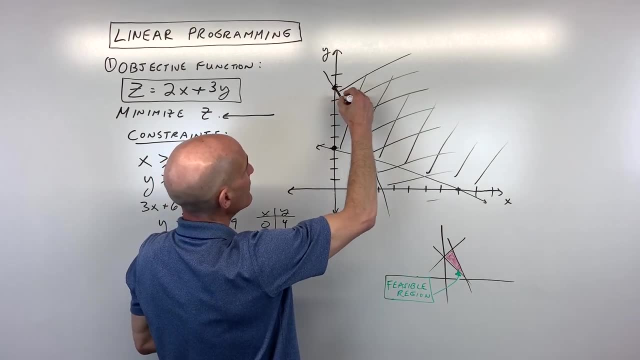 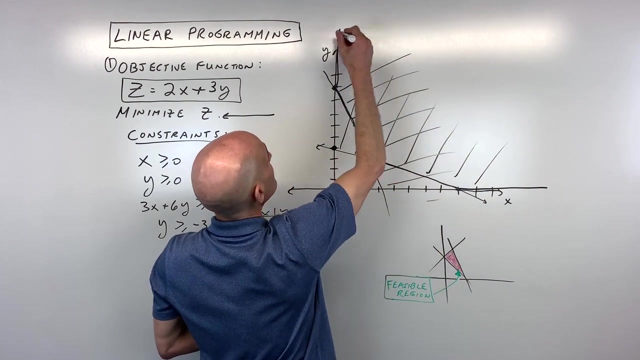 x-axis, we were to the right of the y-axis. we're above this line and we're above this line. So what happens here is that where do all these regions overlap? Well, they're overlapping right here, here, here, and like this. So basically, if I kind of go back and shade this a little bit, 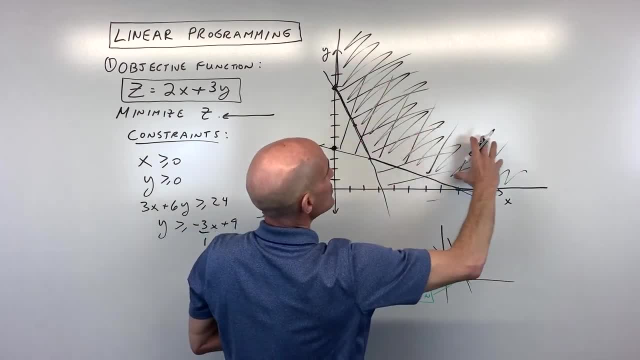 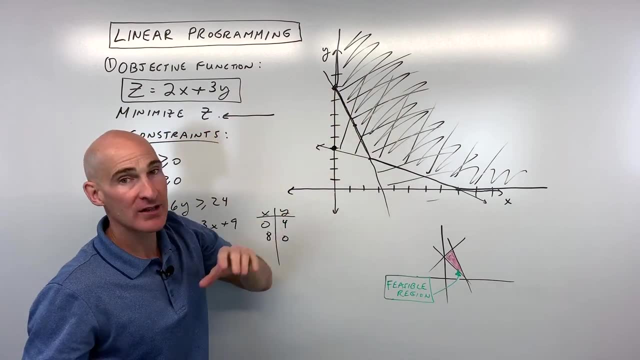 darker here it's going to put us in this region, here. Now, this is what's referred to as an unbounded region, because you can see it keeps going like this, keeps going over like that, and so, you know, continues forever and ever. But what we're going to do now is we're going to pick the. 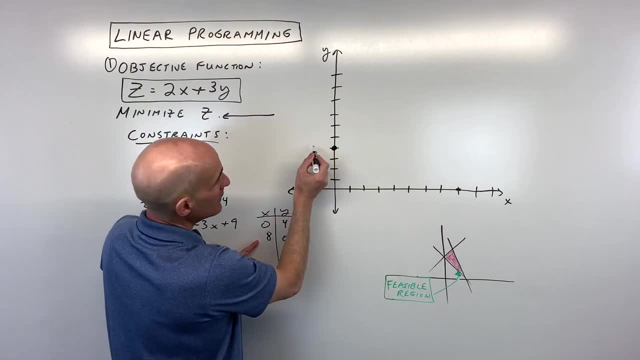 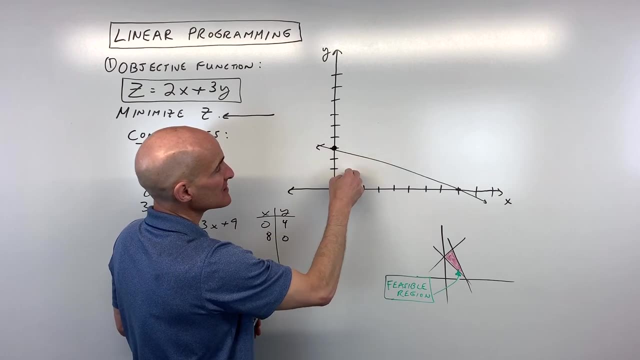 And I'm just going to draw a solid line because it's equal to. and then when you graph using the x and y intercepts like this, you want to pick a point on either side of this line and test it to see if it makes it true. So, for example, if I put 0, 0 in 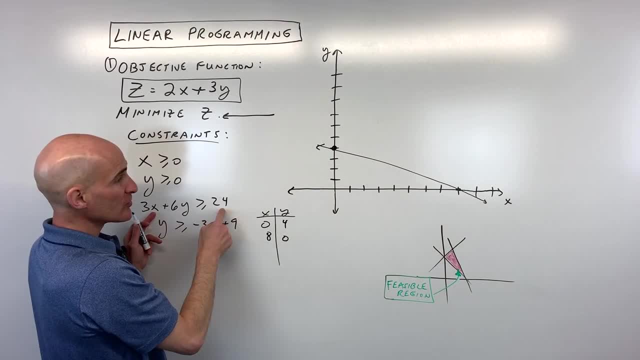 that's the origin. this test point here is 0 greater than or equal to 24? Well, no, So that's means we wouldn't want to shade on this side of the line. we want to shade on this side of the. 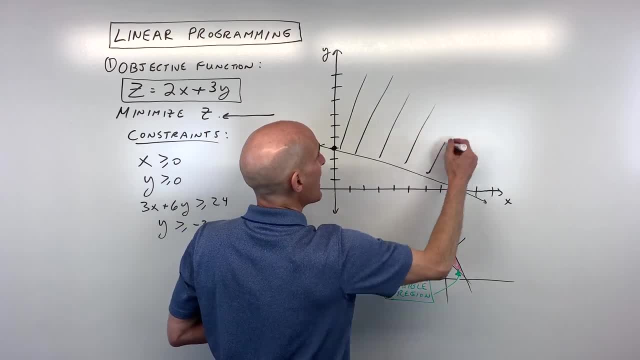 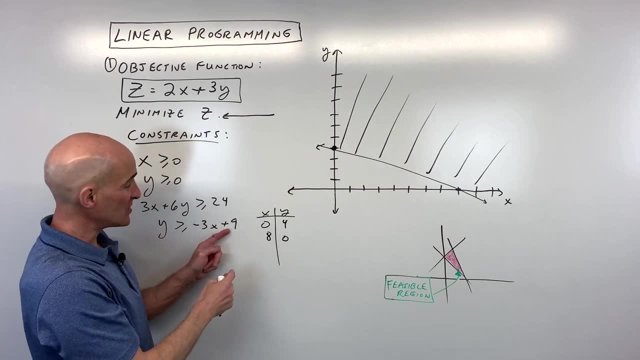 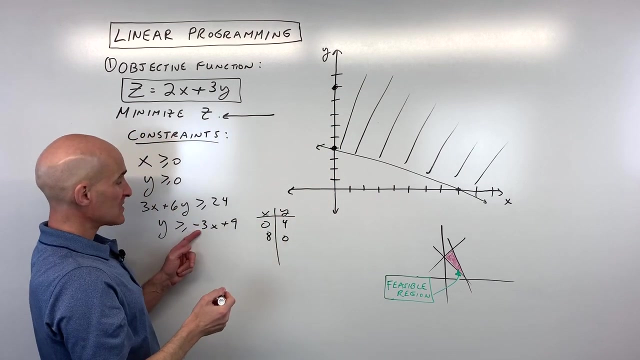 line. So let me go ahead and just draw some lines, just so we know that we're on this side. Okay, for the second inequality, y is greater than or equal to negative 3x plus 9.. So we see that the y intercept is 9, so that's going to be 1,, 2,, 3,, 4,, 5,, 6,, 7,, 8,, 9.. The slope is negative: 3,. 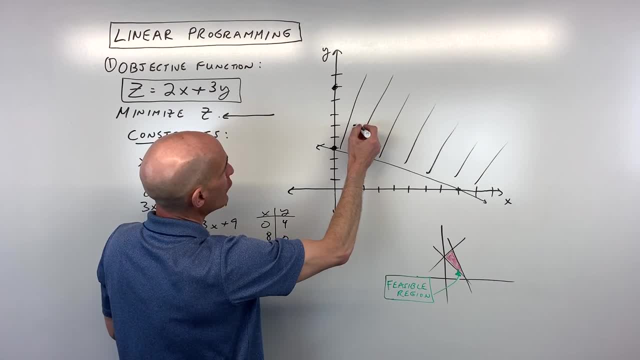 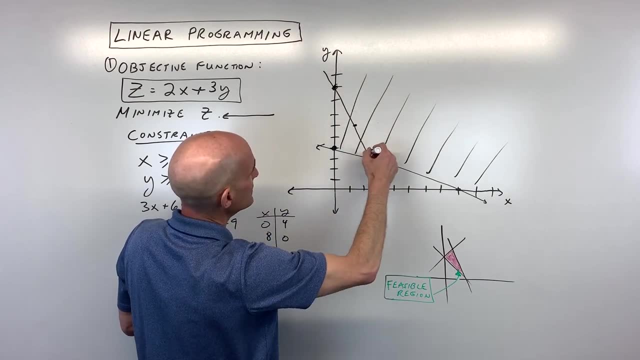 which is like negative 3 over 1, so we're going to go down 3 over 1,, down 3 over 1, so let me just kind of draw this in. Okay, something like that. And this one y is by: 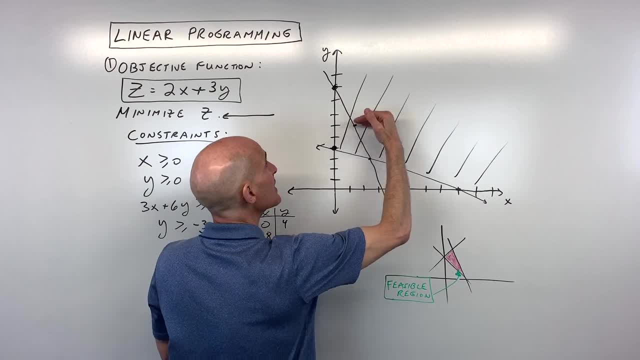 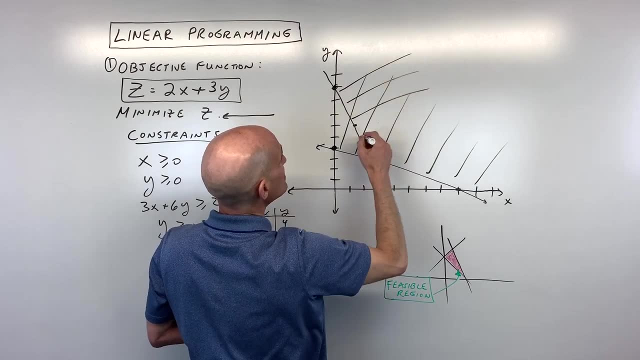 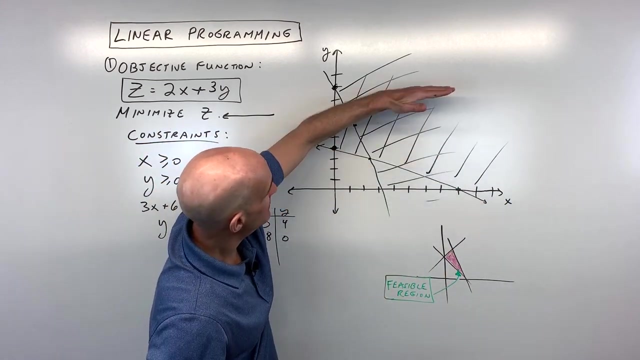 itself and when y is greater than that means that we're going to be shading above the line. So what that means is I'm going to be shading on this side of the line. So let me just draw some lines just to illustrate some shading here. Okay, like that. Now you can see that we were above the 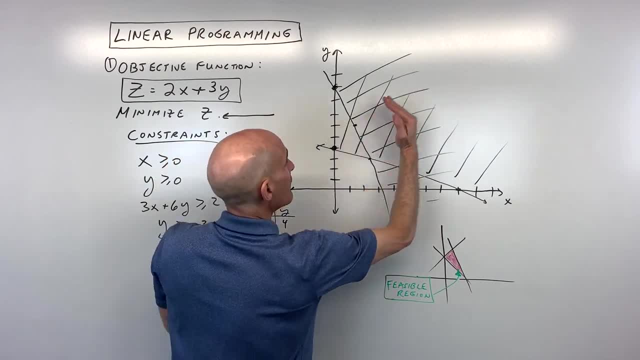 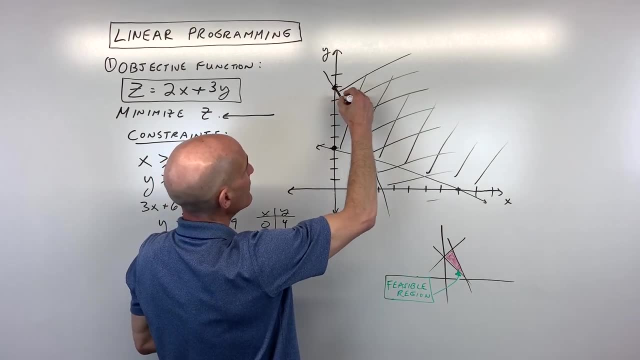 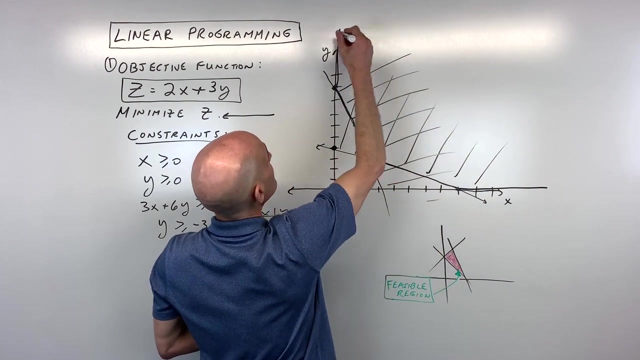 x-axis, we were to the right of the y-axis. we're above this line and we're above this line. So what happens here is that where do all these regions overlap? Well, they're overlapping right here, here, here, and like this. So basically, if I kind of go back and shade this a little bit, 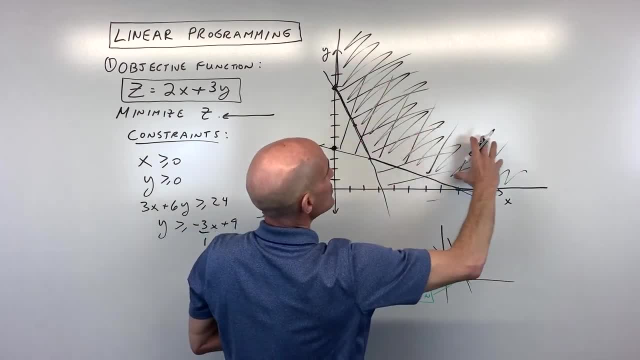 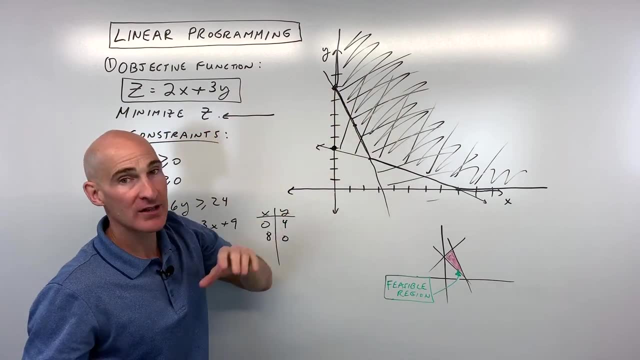 darker here it's going to put us in this region, here. Now, this is what's referred to as an unbounded region, because you can see it keeps going like this, keeps going over like that, and so, you know, continues forever and ever. But what we're going to do now is we're going to pick the. 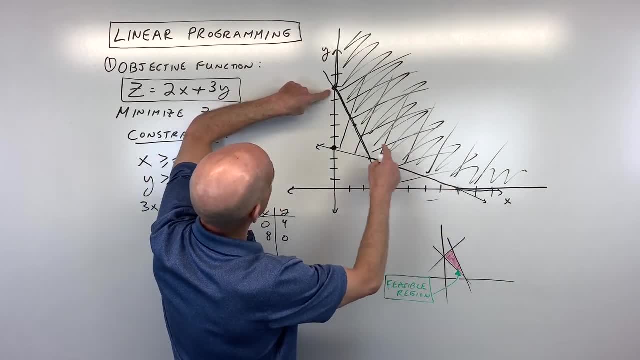 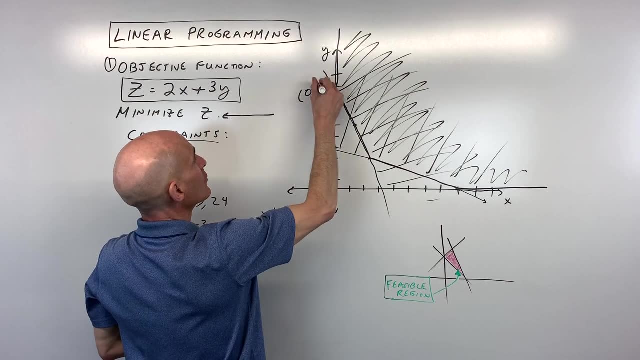 points, these vertices along this region here. So we're going to take this point here, which was the point. let's see one, two, three, four, five, six, seven, eight, nine, so zero, nine, We're going. 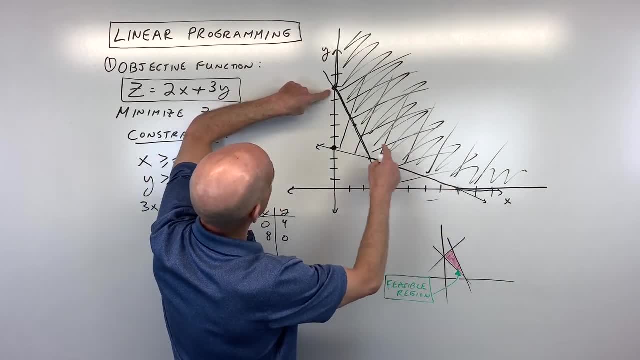 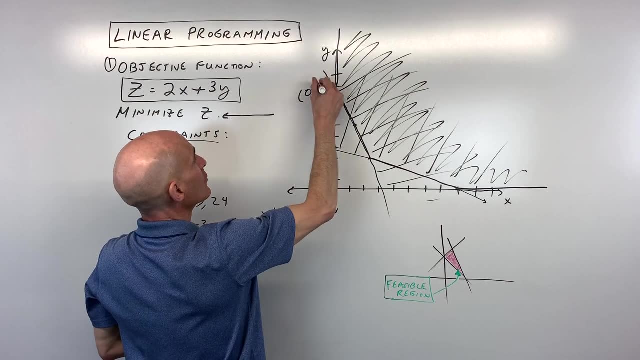 points, these vertices along this region here. So we're going to take this point here, which was the point. let's see one, two, three, four, five, six, seven, eight, nine, so zero, nine, We're going. 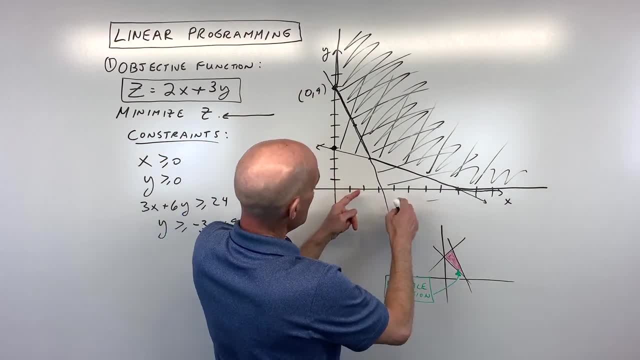 to take this point here, which we're going to solve for in a minute, and then we're going to take this point here, which is: one, two, three, four, five, six, seven, eight comma zero. Now, how do we? 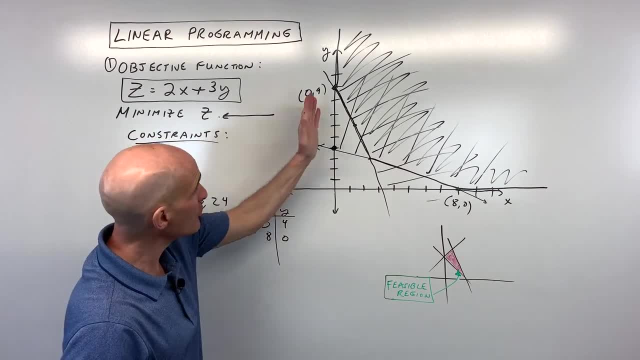 find this point here. This is probably the toughest part of the problem. Well, remember, this is this line and this is this line, and we're trying to find where they intersect. So that's these two lines here. So what we're going to do is we're going to take this point here and we're going to 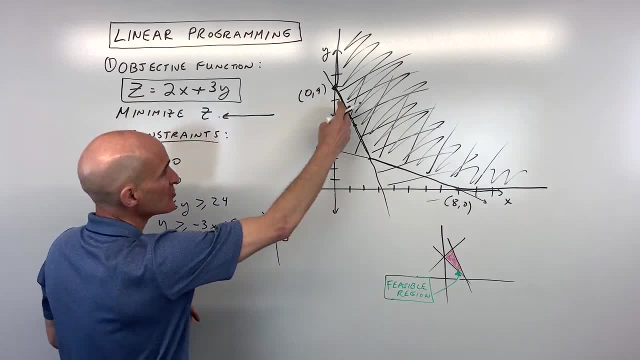 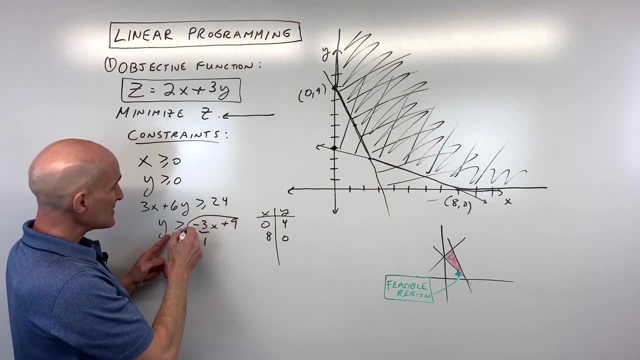 do is we're going to treat them like equations, not inequalities. Now, we're just going to treat them like lines. We want to find the intersection point, and I think the easiest way to do this one is to use substitution. So if y is equal to negative 3x plus 9, let's put that in place of y. 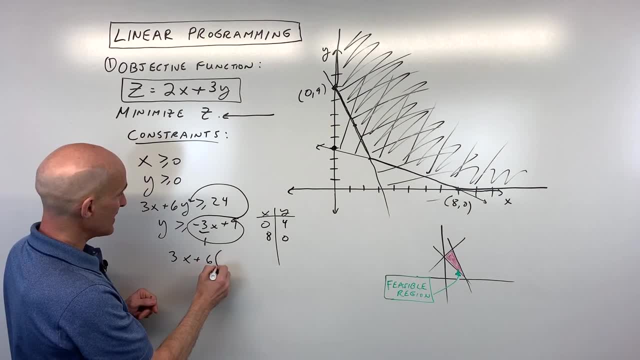 here in this equation. So we get 3x plus 6 times negative. 3x plus 9 is equal to 24.. So let's go ahead and solve this. Distribute That gives us negative 18x plus 54.. Bring down the three. 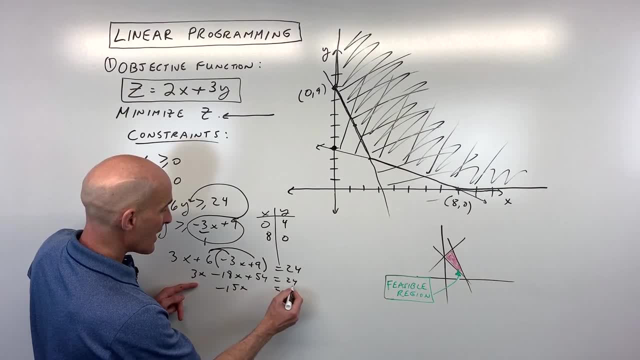 x, This comes out to negative 15x. Subtract the 54. That's negative 30, and divide both sides by negative 15, and x is equal to 2.. Now if we take 2 and we put it back in here, you get negative 3. 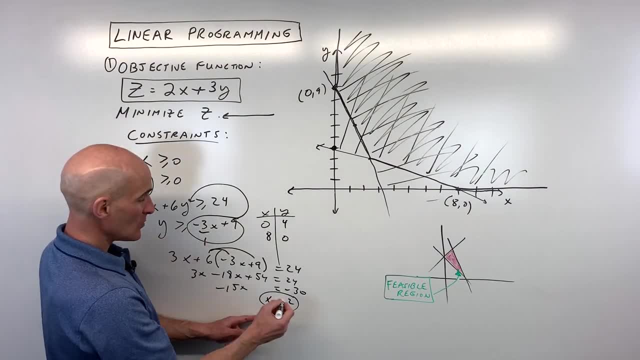 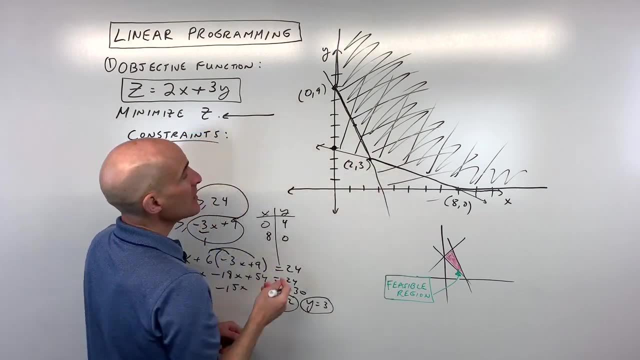 times 2 is negative 6, plus 9 is 3.. So you can see y is equal to 3, and that's the coordinates of this point right here: 2 comma 3.. So now, what we're going to do is we're going to take these: 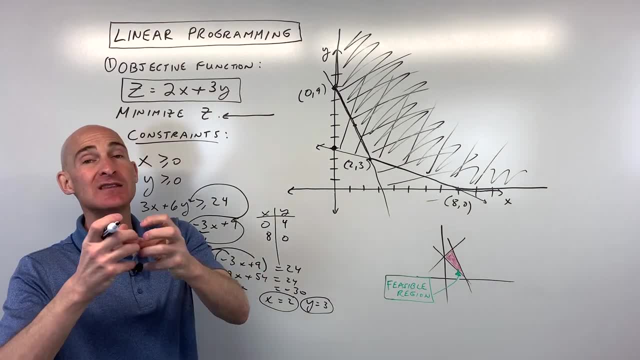 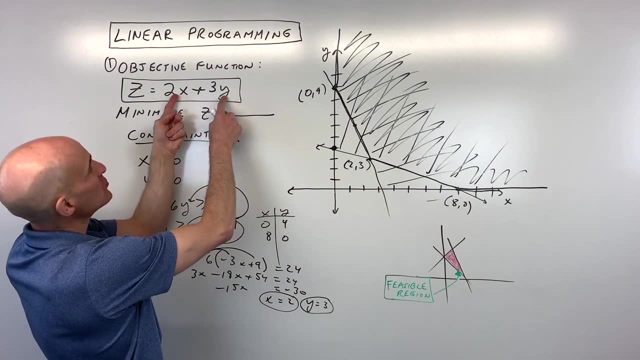 vertices, put them into our objective function and see which one gives us the minimum value, the smallest value. So let's go ahead and put 0 in for x, 9 in for y, So that's going to be 2 times. 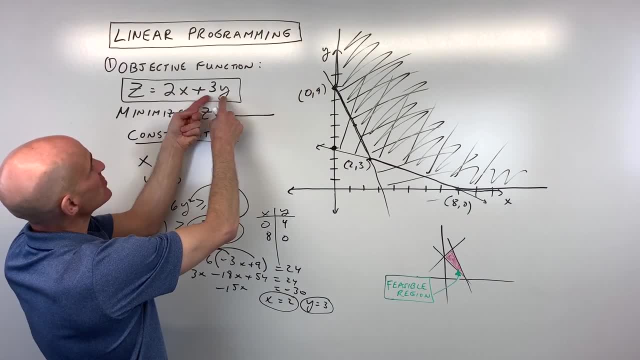 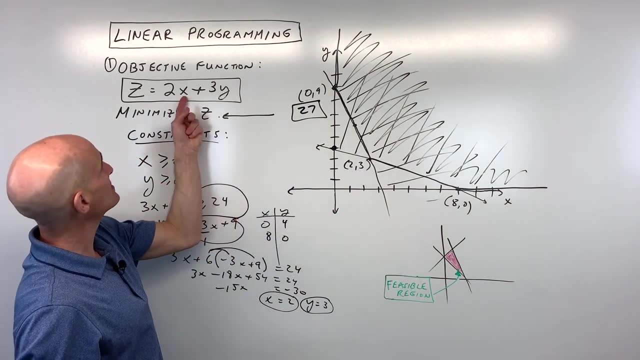 0, which is 0.. 3 times 9 is 27.. 0 plus 27 is 27.. So for this point we get a value of 27.. Let's put in 2 and 3.. So 2 for x, 2 times 2 is 4.. 3 times 3 is 9.. 4 plus 9 is 13.. Okay, at that point, And 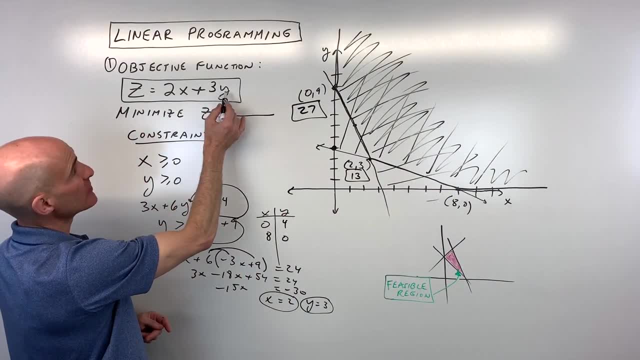 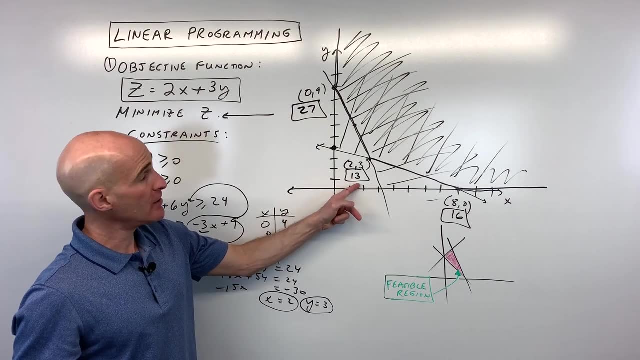 then if we pick 8, 0.. 2 times 8 is 16.. 3 times 0 is 0.. 16 plus 0 is 16.. So which one gave us the minimum value? It looks like this one right here: 13.. 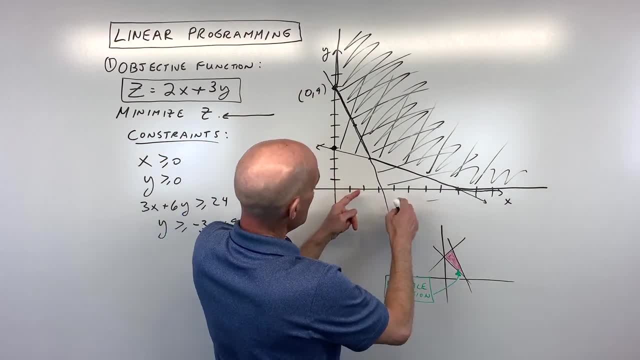 to take this point here, which we're going to solve for in a minute, and then we're going to take this point here, which is: one, two, three, four, five, six, seven, eight comma zero. Now, how do we? 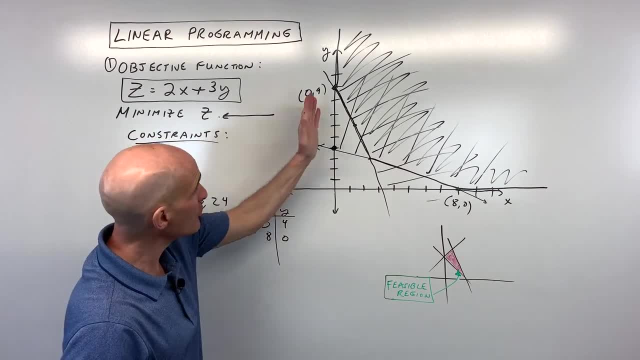 find this point here. This is probably the toughest part of the problem. Well, remember, this is this line and this is this line, and we're trying to find where they intersect. So that's these two lines here. So what we're going to do is we're going to take this point here and we're going to 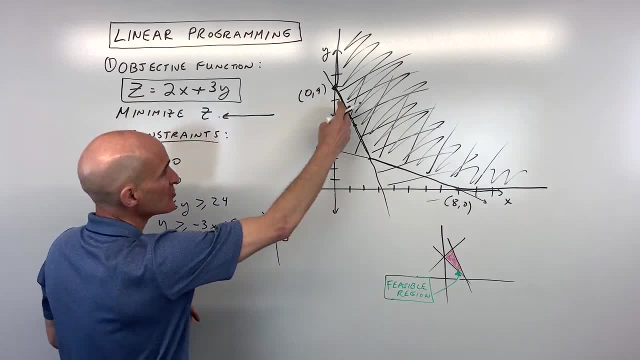 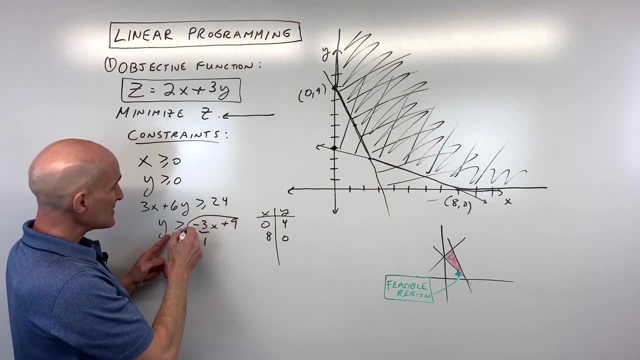 do is we're going to treat them like equations, not inequalities. Now, we're just going to treat them like lines. We want to find the intersection point, and I think the easiest way to do this one is to use substitution. So if y is equal to negative 3x plus 9, let's put that in place of y. 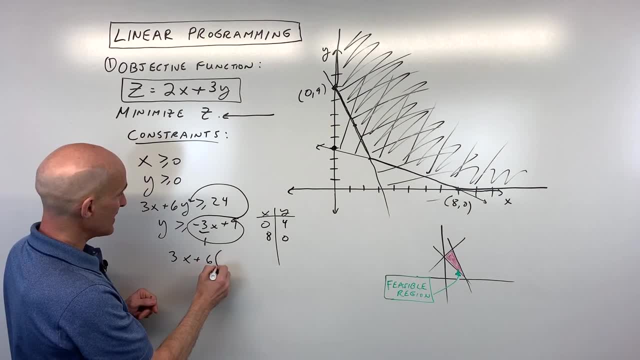 here in this equation. So we get 3x plus 6 times negative. 3x plus 9 is equal to 24.. So let's go ahead and solve this. Distribute That gives us negative 18x plus 54.. Bring down the three. 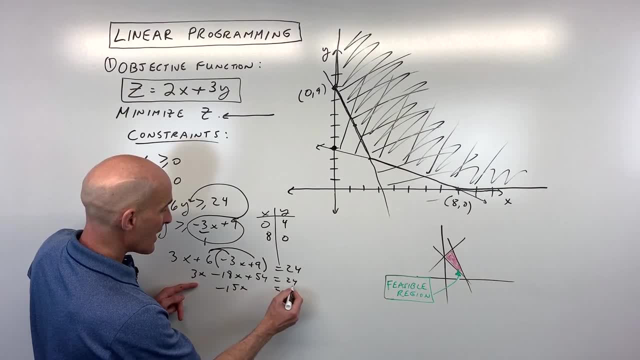 x, This comes out to negative 15x. Subtract the 54. That's negative 30, and divide both sides by negative 15, and x is equal to 2.. Now if we take 2 and we put it back in here, you get negative 3. 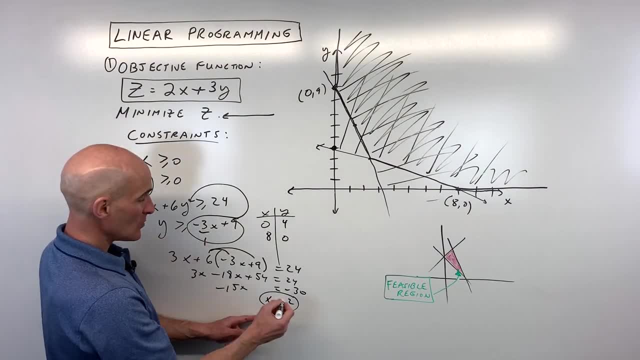 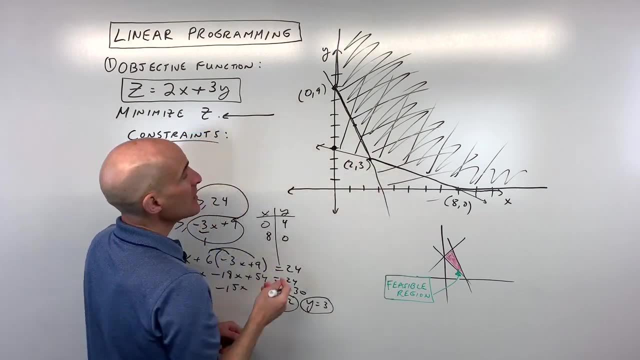 times 2 is negative 6, plus 9 is 3.. So you can see y is equal to 3, and that's the coordinates of this point right here: 2 comma 3.. So now, what we're going to do is we're going to take these: 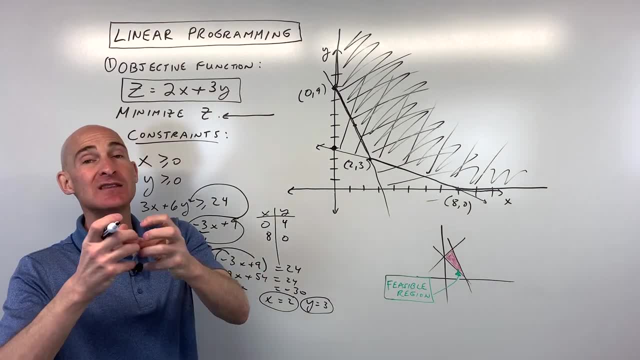 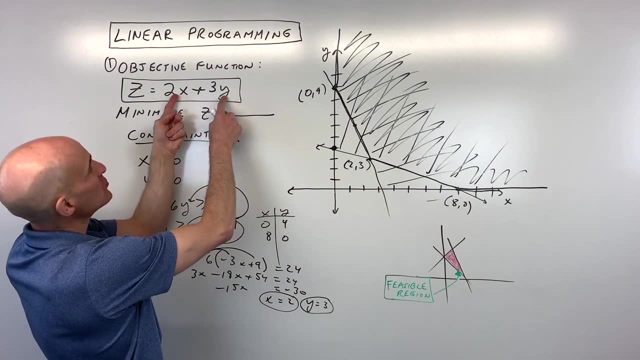 vertices, put them into our objective function and see which one gives us the minimum value, the smallest value. So let's go ahead and put 0 in for x, 9 in for y, So that's going to be 2 times. 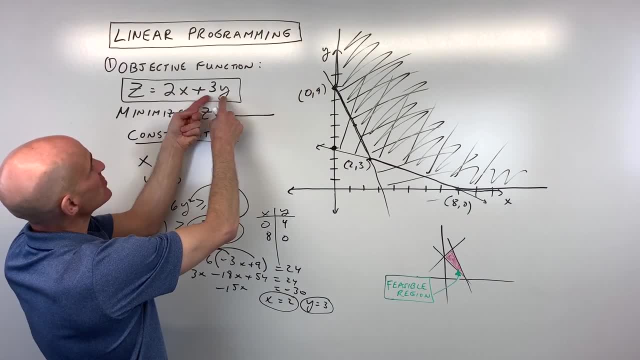 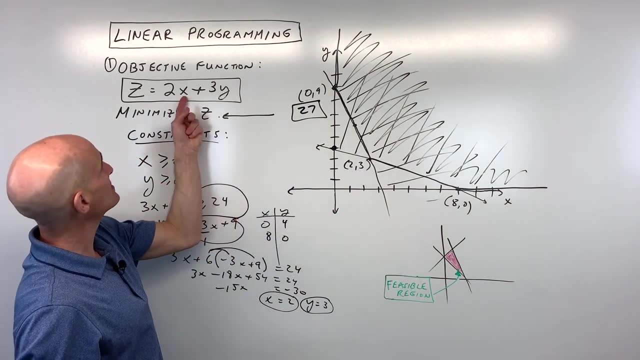 0, which is 0.. 3 times 9 is 27.. 0 plus 27 is 27.. So for this point we get a value of 27.. Let's put in 2 and 3.. So 2 for x, 2 times 2 is 4.. 3 times 3 is 9.. 4 plus 9 is 13.. Okay, at that point, And 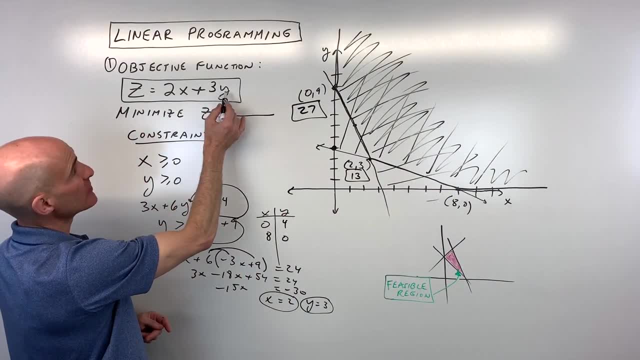 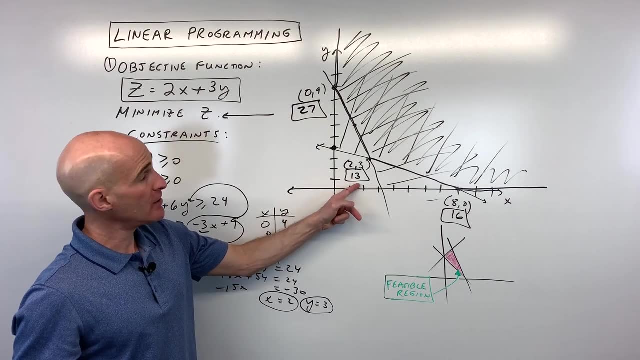 then if we pick 8, 0.. 2 times 8 is 16.. 3 times 0 is 0.. 16 plus 0 is 16.. So which one gave us the minimum value? It looks like this one right here: 13.. 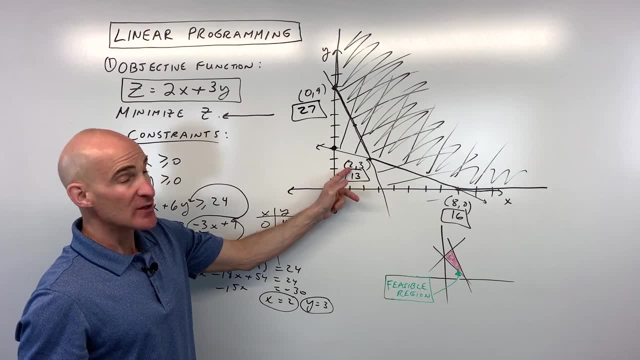 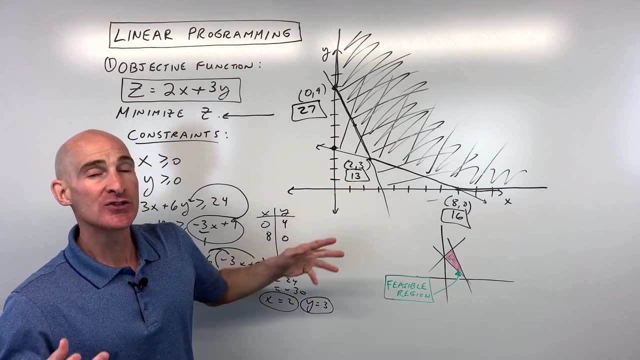 So to minimize, you would want there to be 2 of whatever the x quantity is, 3 of whatever the y quantity is, and that's going to give you a minimum value of 13.. So let's go ahead and dive into a word problem now, where we're going to maximize the profit, Before we dive into this. 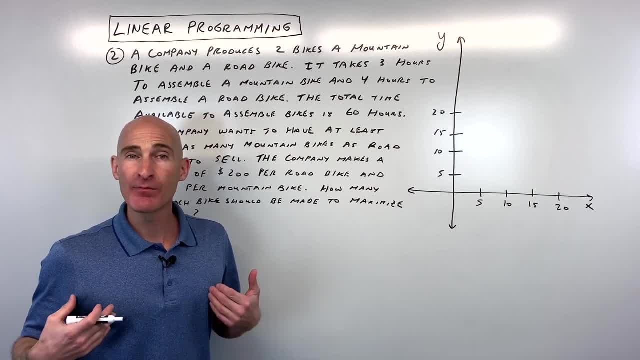 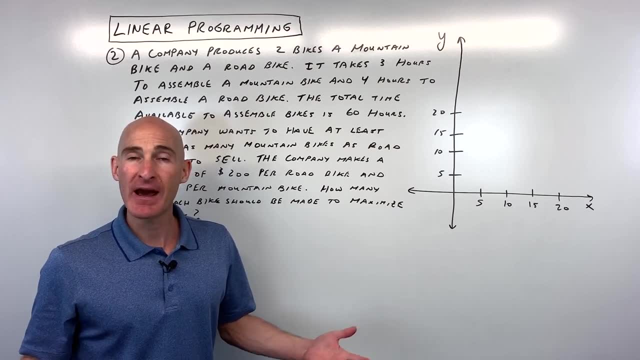 word problem if you're new to the channel and we haven't met yet. my name is Mario of Mario's Math Tutoring, and my goal for this channel is to make learning math less stressful, so that you can raise your grade, pass your class and go on to pursue your dreams. So I'm a full-time. 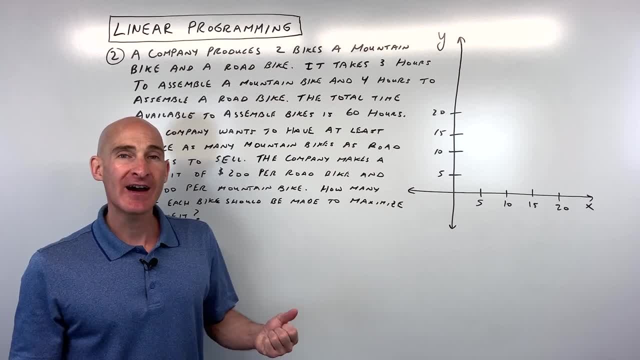 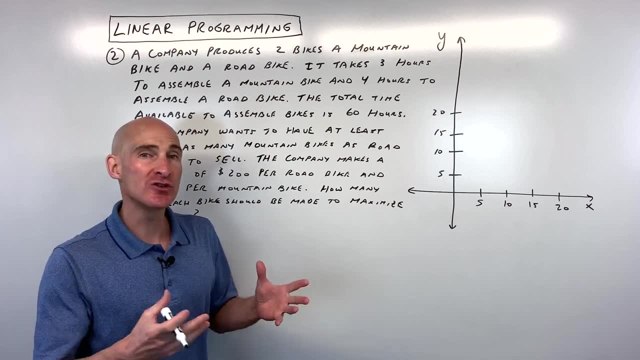 math tutor. I work with students every day and what I do is I try to find the simplest and easiest and most understandable way to do some of these problems and I take it and try to condense it down and put it into these videos so that you can benefit from my tutoring as well. So if that's, 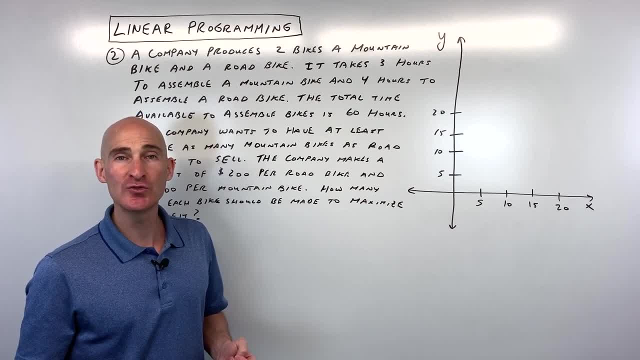 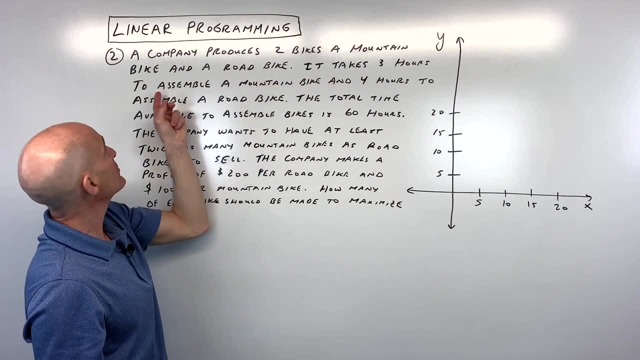 something you're interested in. check out more videos on my Mario's Math Tutoring YouTube channel. But let's dive into number two. A company produces two bikes: a mountain bike and a road bike. It takes three hours to assemble a mountain bike and takes four hours to assemble a road bike. 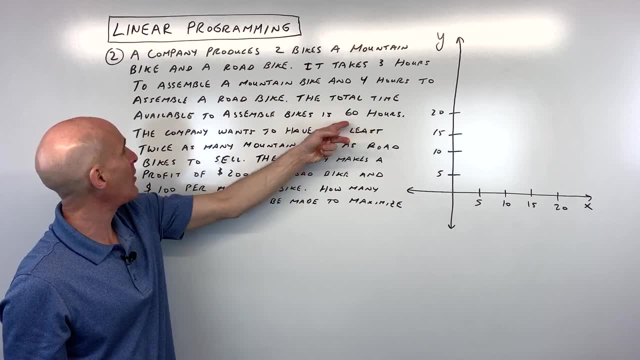 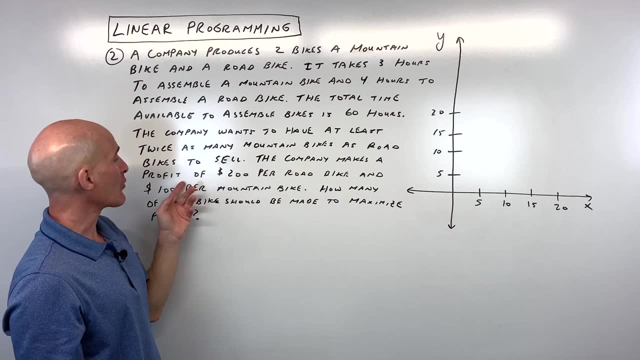 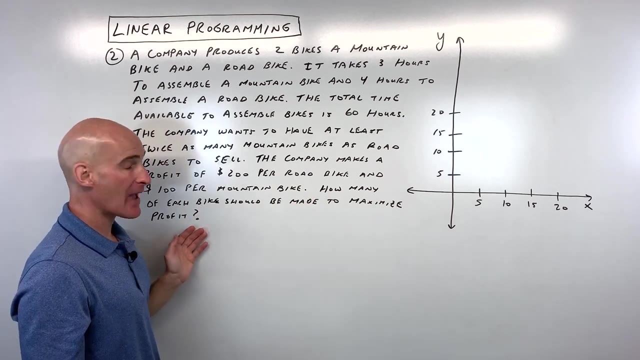 The total time available to assemble bikes is 60 hours. The company wants to have at least twice as many mountain bikes as road bikes to sell. The company makes a profit of $200 per road bike and $100 per mountain bike. How many of each bike should be made to maximize the profit? 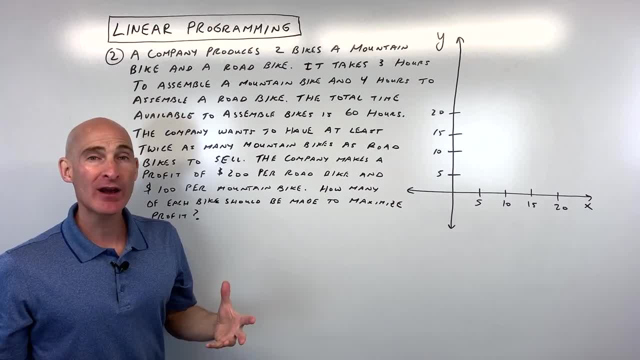 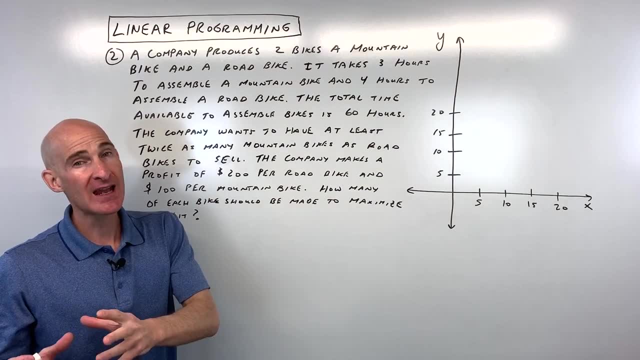 So that's kind of a lot of words there, And usually what I recommend when you're doing these story problems is just kind of read through it real quickly. You don't have to get everything the first time. And then usually what you want to focus on on these optimization, these linear programming problems, is the last sentence. 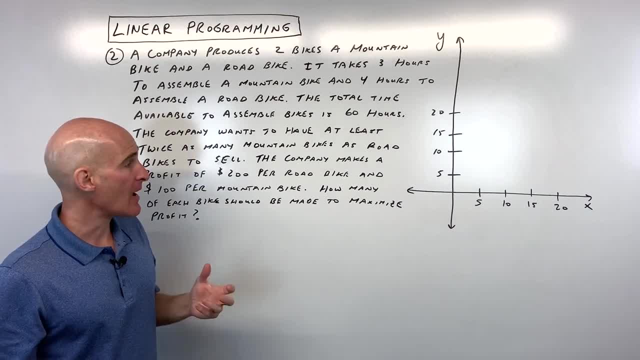 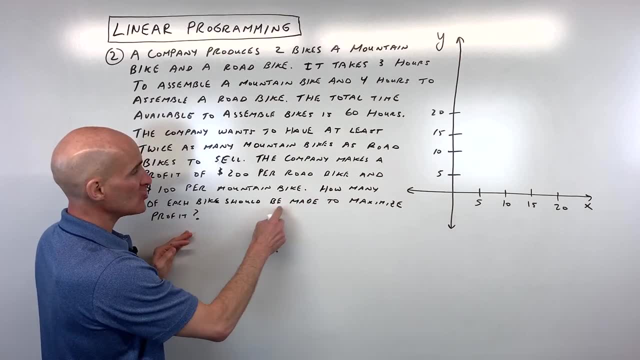 That'll usually tell you the story as far as what you're looking to maximize or minimize, And it'll also tell you what your variables are. So let's do that. So it says how many of each bike should be made to maximize the profit. 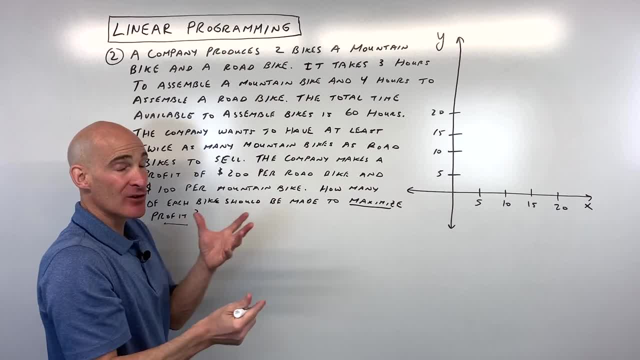 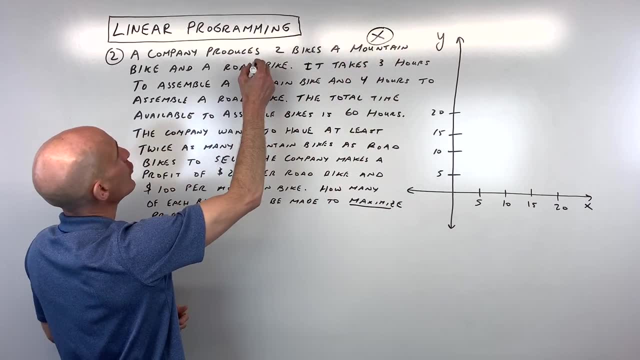 So we know we're trying to maximize profit And we're trying to figure out how many road bikes And how many mountain bikes. So why don't we call the mountain bikes X And we're going to call the road bikes Y? Okay, so on our graph here I'm just going to say X is mountain bikes. 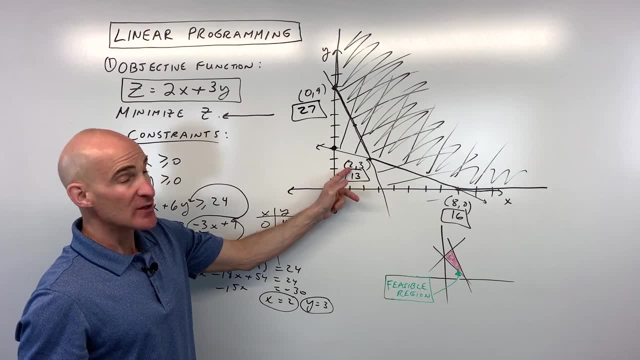 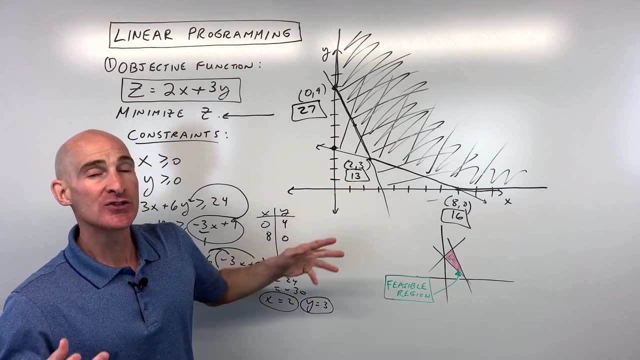 So to minimize, you would want there to be 2 of whatever the x quantity is, 3 of whatever the y quantity is, and that's going to give you a minimum value of 13.. So let's go ahead and dive into a word problem now, where we're going to maximize the profit, Before we dive into this. 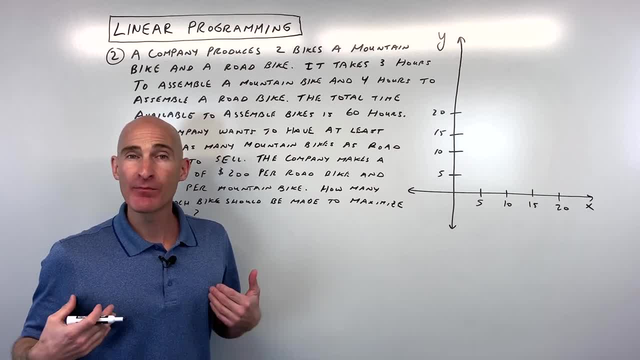 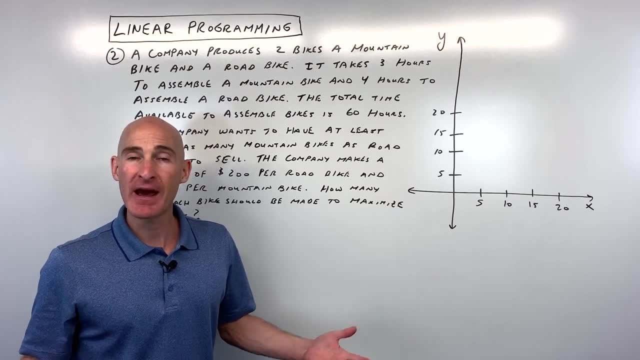 word problem if you're new to the channel and we haven't met yet. my name is Mario of Mario's Math Tutoring, and my goal for this channel is to make learning math less stressful, so that you can raise your grade, pass your class and go on to pursue your dreams. So I'm a full-time. 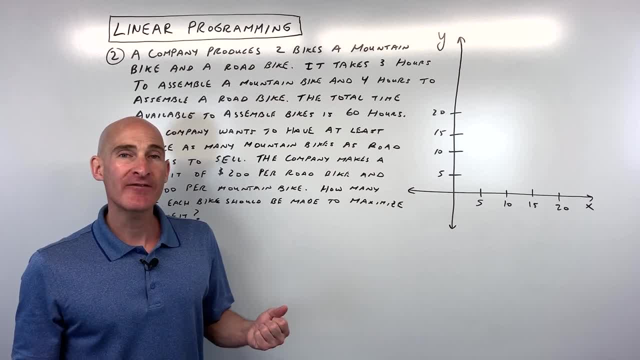 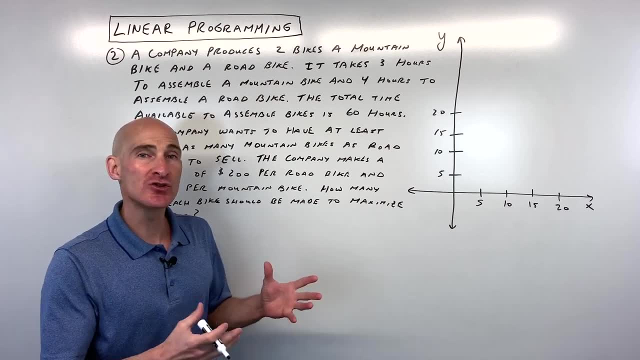 math tutor. I work with students every day and what I do is I try to find the simplest and easiest and most understandable way to do some of these problems And I take it and try to condense it down and put it into these videos so that you can benefit from my tutoring as well. So if that's, 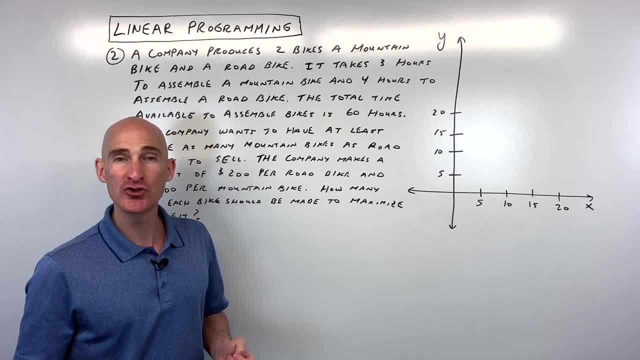 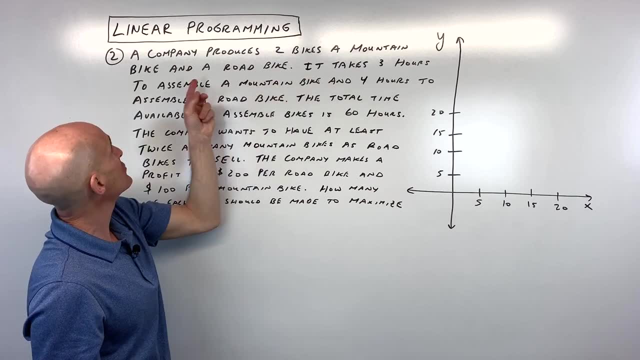 something you're interested in. check out more videos on my Mario's Math Tutoring YouTube channel. but let's dive into number two. A company produces two bikes: a mountain bike and a road bike. It takes three hours to assemble a mountain bike and takes four hours to assemble a road bike. 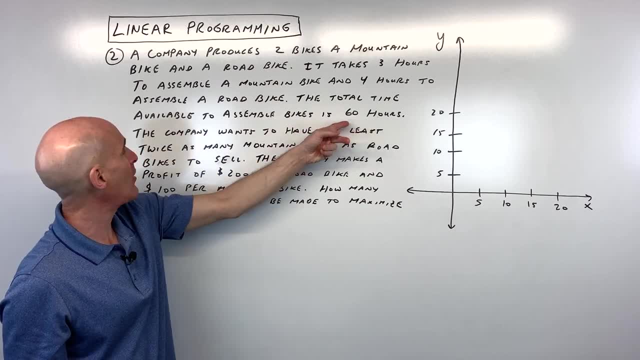 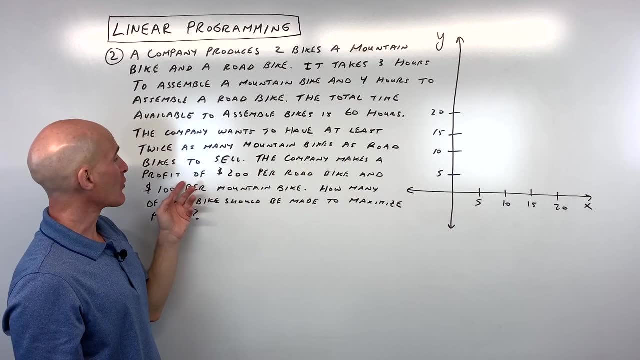 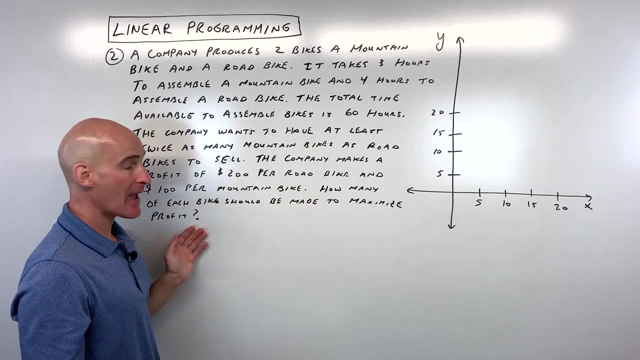 The total time available to assemble bikes is 60 hours. The company wants to have at least twice as many mountain bikes as road bikes to sell. The company makes a profit of $200 per road bike and $100 per mountain bike. How many of each bike should be made to maximize the profit? So 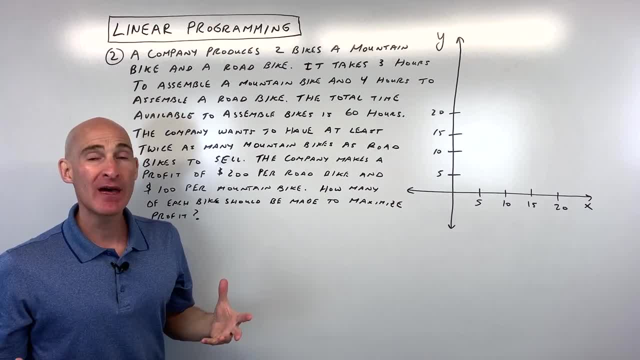 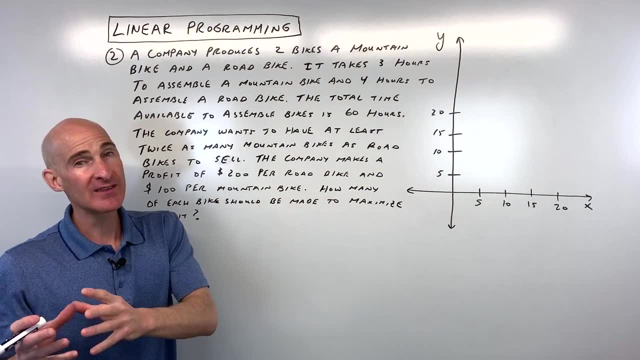 that's kind of a lot of words there, And usually what I recommend when you're doing these story problems is just kind of read through it real quickly- You don't have to get everything the first time- And then usually what you want to focus on, on these optimization, these linear 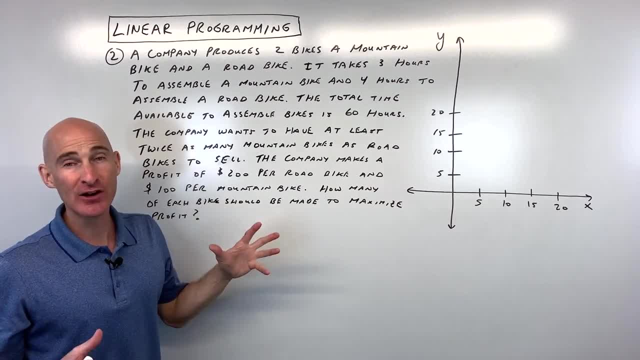 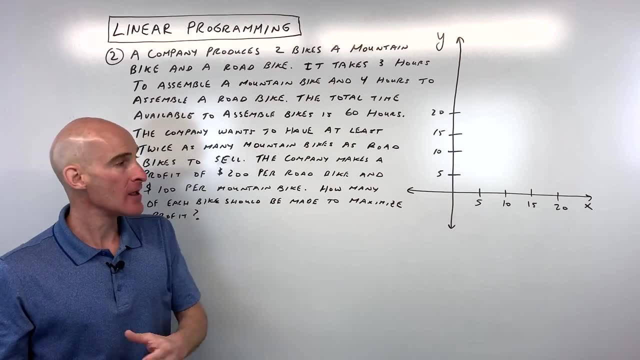 programming problems is the last sentence. That'll usually tell you the story as far as what you're looking to maximize or minimize, And it'll also tell you what your variables are. So let's do that. So it says how many of each bike should be made to maximize the profit. So we know we're. 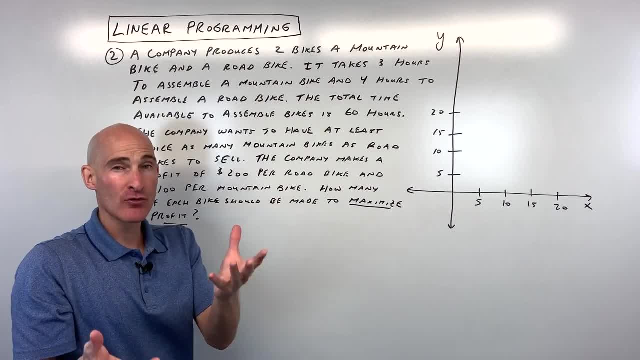 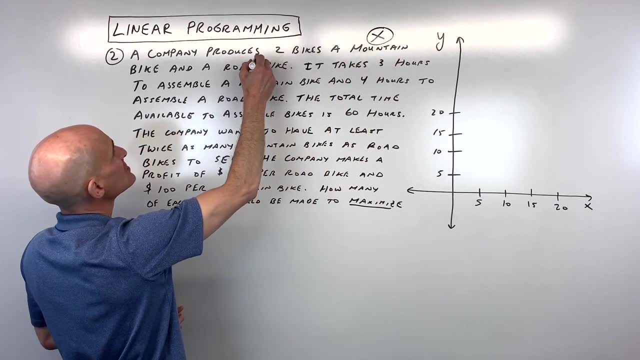 trying to maximize profit And we're trying to figure out how many road bikes and how many mountain bikes. So why don't we call the mountain bikes X and we're going to call the road bikes Y? Okay, so on our graph here, I'm just 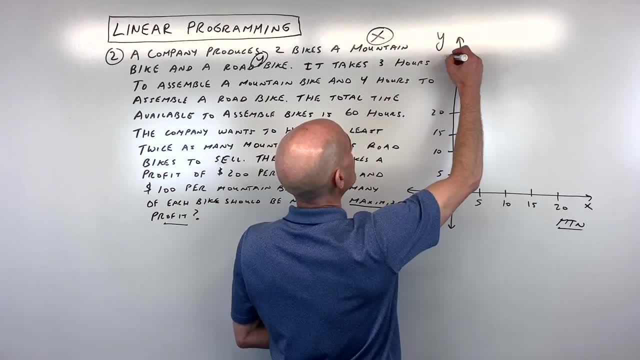 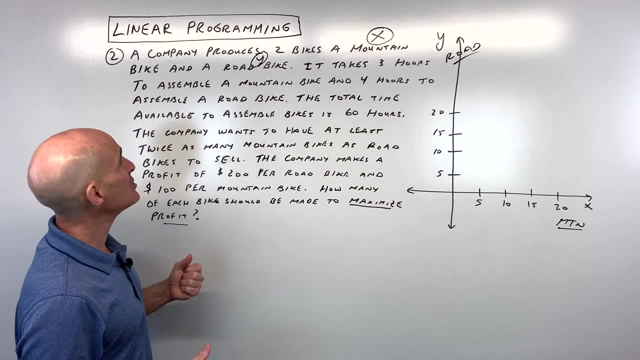 going to say X is mountain bikes and Y, over here, is going to be the road bikes. Okay, so now let's look at what are called the constraints. These are our restrictions, our limitations. See how it says: it takes three hours to assemble a mountain bike and four hours to assemble a road bike. but you 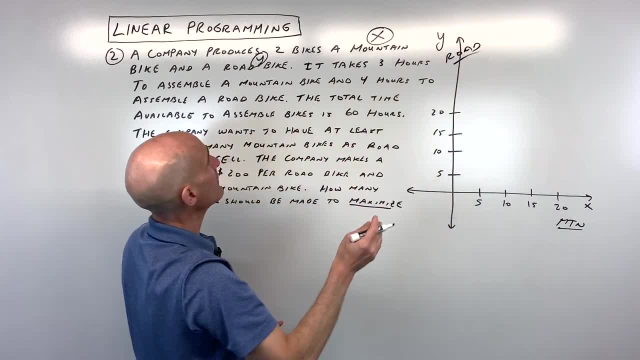 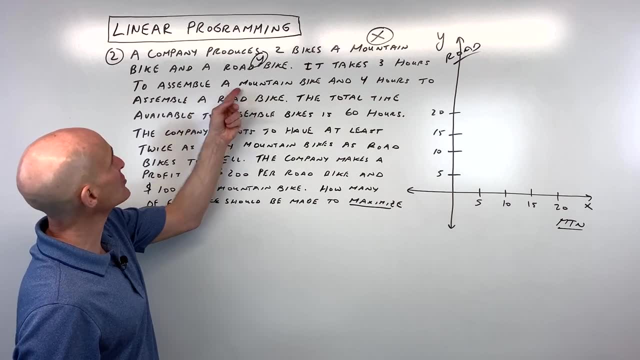 And Y over, here is going to be the road bikes. Okay, so now let's look at what are called the constraints. These are our restrictions, our limitations. See how it says: it takes three hours to assemble a mountain bike and four hours to assemble a road bike. 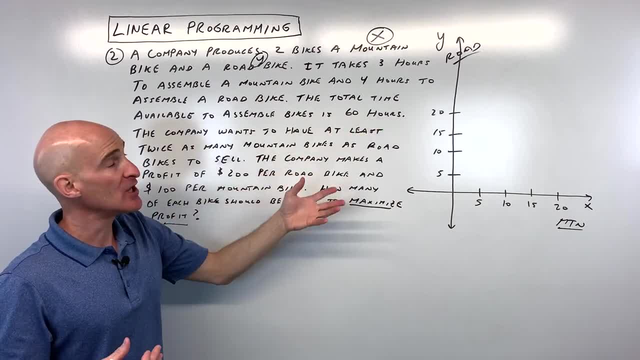 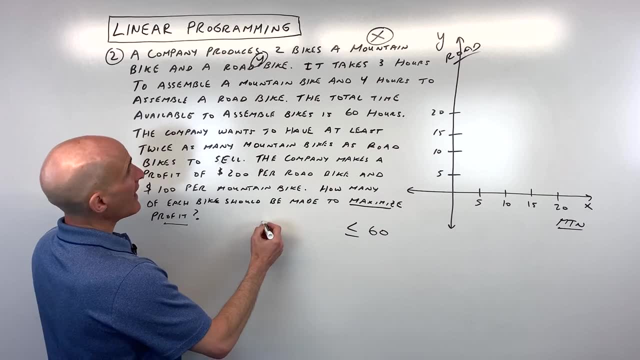 But you only have 60 hours available. So can you work more than 60? No, it has to be less than or equal to 60.. So we've got three hours to assemble a mountain bike. We have four hours to assemble a road bike. 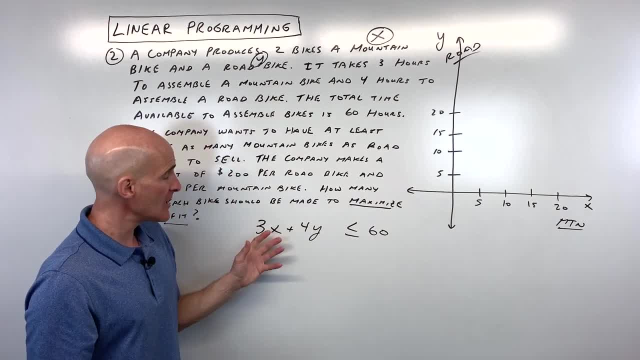 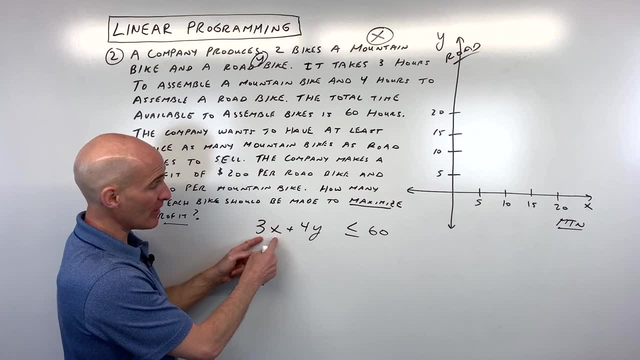 But the amount of time spent assembling has to be less than or equal to 60 hours. Now notice like: see, if you assembled like four mountain bikes, Well, four times three hours per mountain bike, that's 12 hours assembling mountain bikes, right. 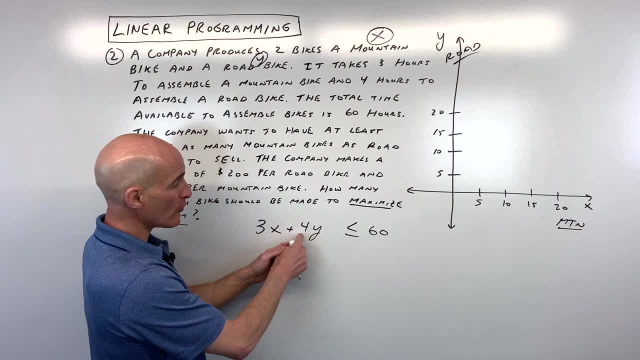 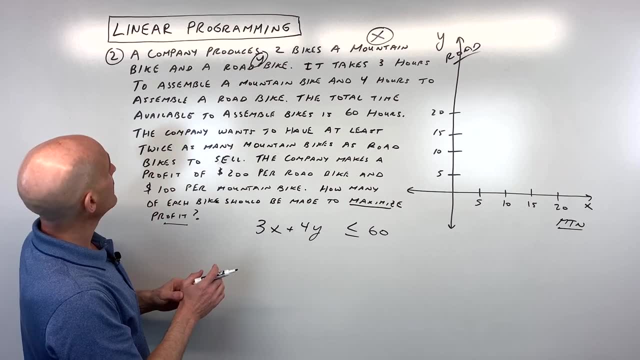 Or if you did five road bikes five times four hours to assemble one road bike, that's 20 hours spent And you want to make sure that total is less than or equal to 60.. Now, what other constraints are there? Well, we know that you can't assemble like a negative number of bikes, right? 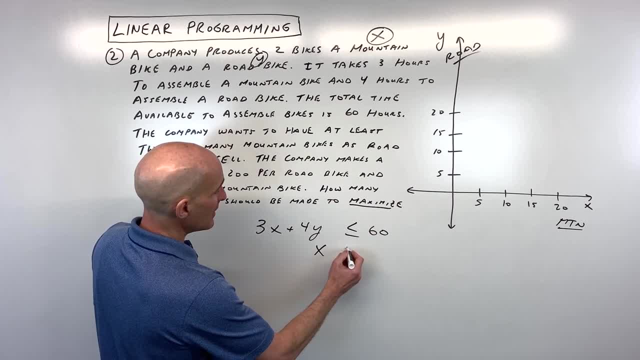 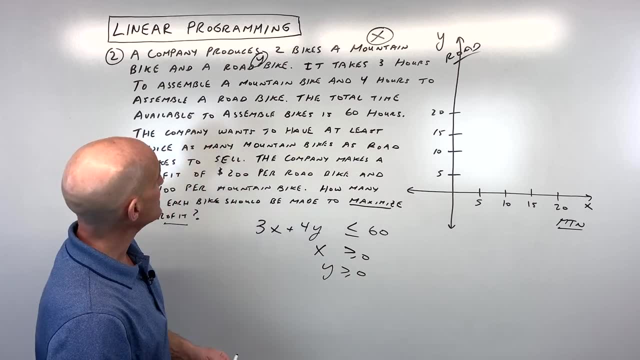 So, right off the bat, we know that x has to be greater than or equal to zero. The number of mountain bikes and the number of road bikes also has to be greater than zero. So what that does is it puts us, you know, in this first quadrant. 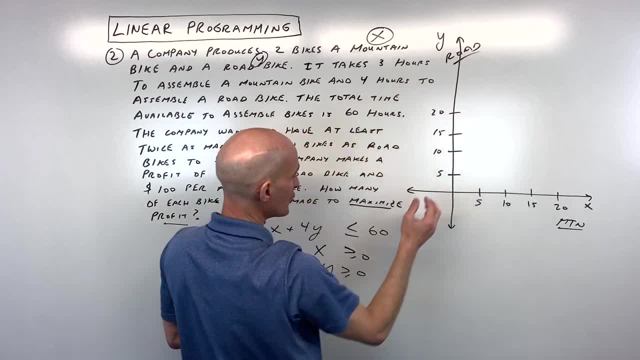 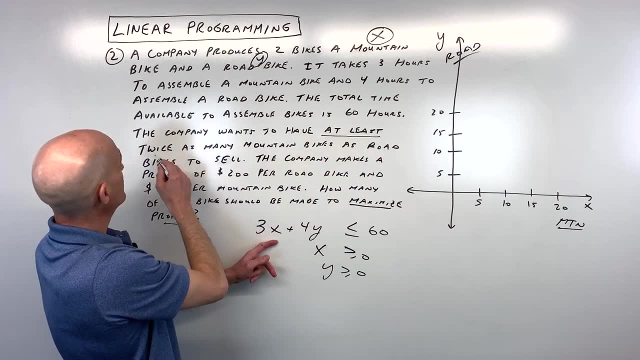 Because x is greater than or equal to zero, Y is greater than or equal to zero. Those are going to overlap in the first quadrant. But we also have one more constraint Here. it says the company wants to have at least twice as many mountain bikes as road bikes to sell right. 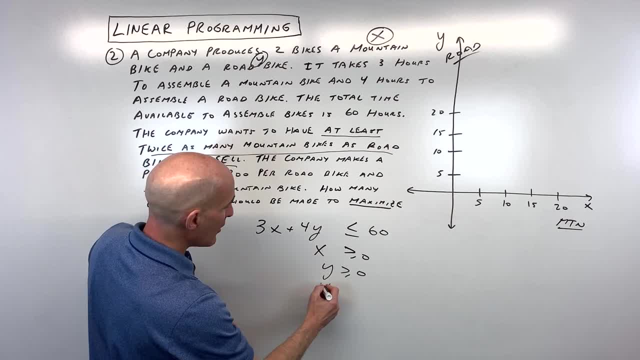 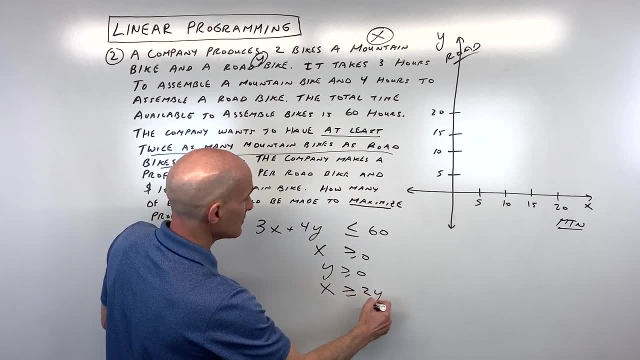 So they want to have at least twice as many mountain bikes. So the number of mountain bikes x has to be at least that's greater than or equal to twice as many road bikes. Okay, so maybe mountain bikes are more popular, right? 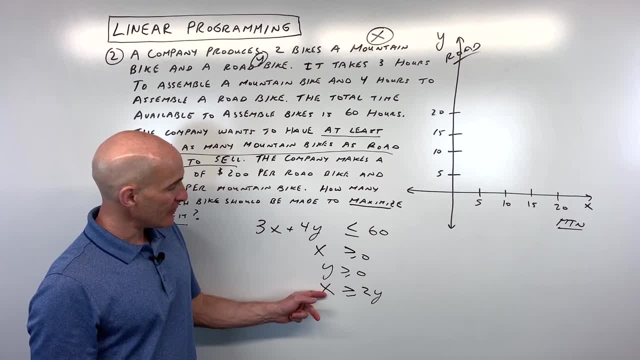 But what's interesting about this inequality is see how we have x by itself. We could rearrange this to get y by itself, But we'll do that in a minute. The first thing we want to do, though, is we want to make sure that x is greater than or equal to zero. 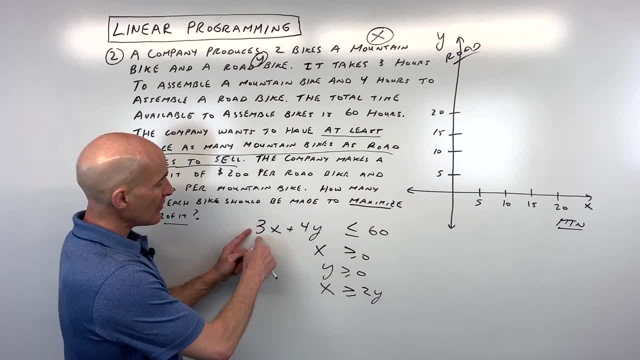 We want to look at a couple different ways to graph these. Like you see how this one's kind of like in the standard form. See how the variables are on the left, numbers on the right. Usually when it's in this form, I like to use the intercept method. 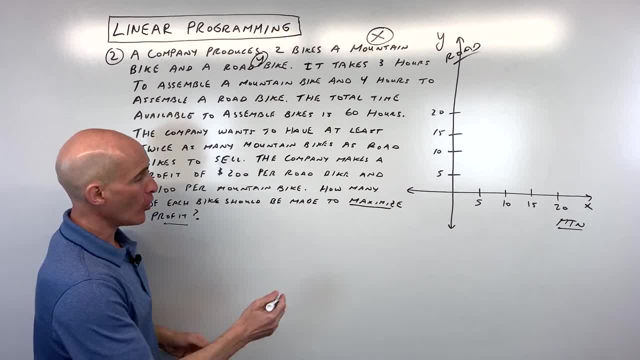 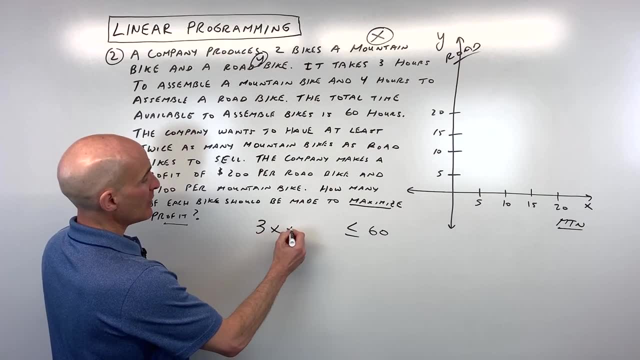 can't do that. So can you work more than 60 hours? No, it has to be less than or equal to 60.. So we've got three hours to assemble a mountain bike. We have four hours to assemble a road bike, but the amount 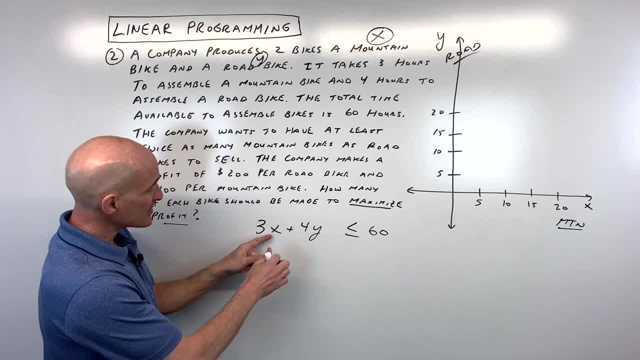 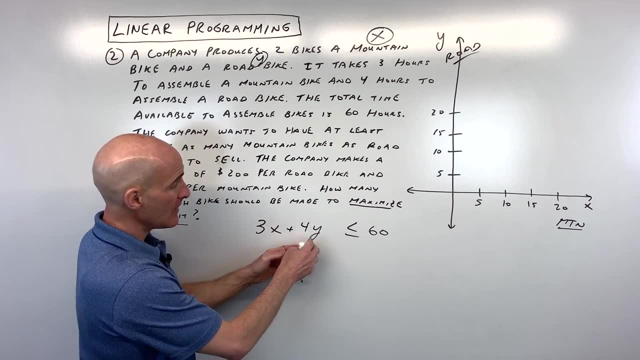 of time spent assembling has to be less than or equal to 60 hours. Now notice like: see, if you assembled like four mountain bikes, Well, four times three hours per mountain bike, that's 12 hours assembling mountain bikes, right? Or if you did five road bikes, five times four hours to. 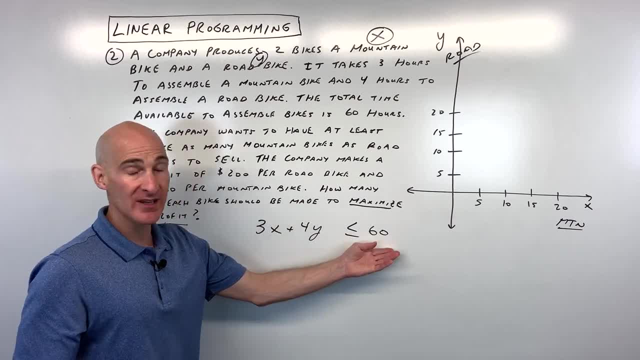 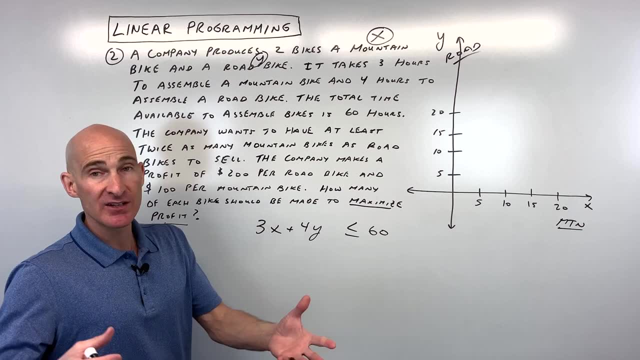 assemble one road bike, that's 20 hours spent. And you want to make sure that you're not doing that because that total is less than or equal to 60. Now, what other constraints are there? Well, we know that you can't assemble like a negative number of bikes, right? So, right off the bat, we know that. 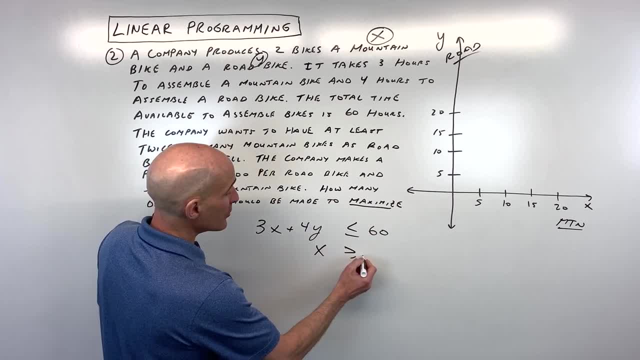 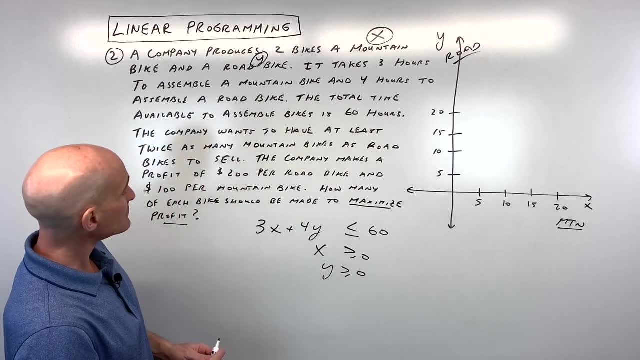 X has to be greater than or equal to zero. the number of mountain bikes and the number of road bikes also has to be greater than or equal to zero. So what that does is it puts us, you know, in this first quadrant, because X is greater than or equal to zero, Y is greater than or equal to zero. 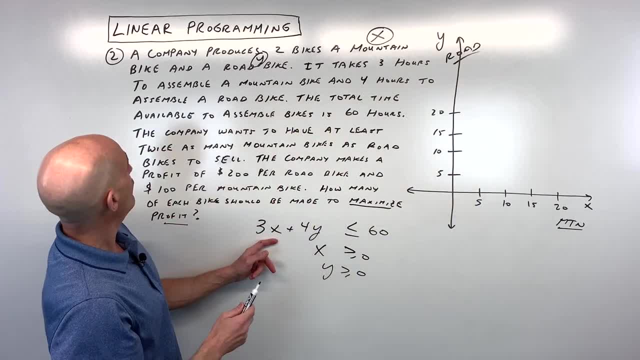 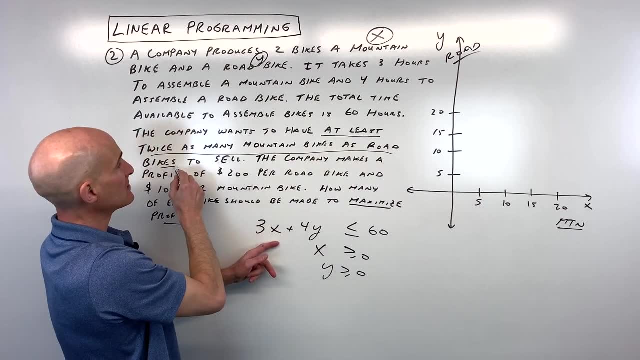 Those are going to overlap in the first quadrant. But we also have one more constraint here. It says the company wants to have at least twice as many mountain bikes as road bikes to sell right. So they want to have at least twice as many mountain bikes. So the number of mountain bikes X has to be. 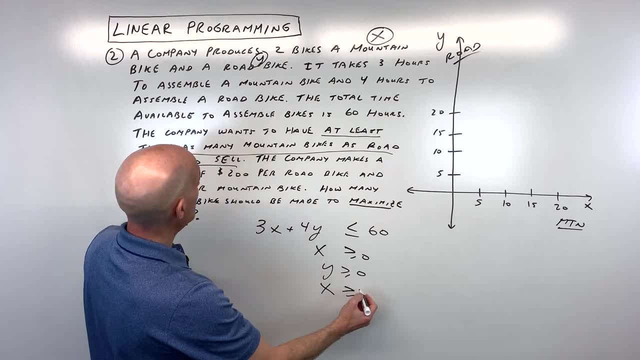 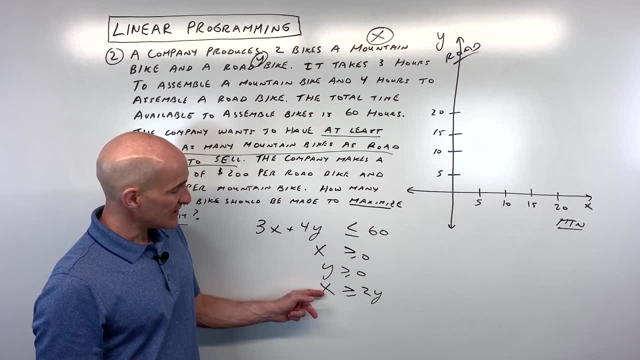 at least that's greater than or equal to twice as many road bikes. Okay, so maybe mountain bikes are more popular, right, But what's interesting about this inequality is see how we have X by itself. We could rearrange that. We could rearrange that. We could rearrange that, We could rearrange. 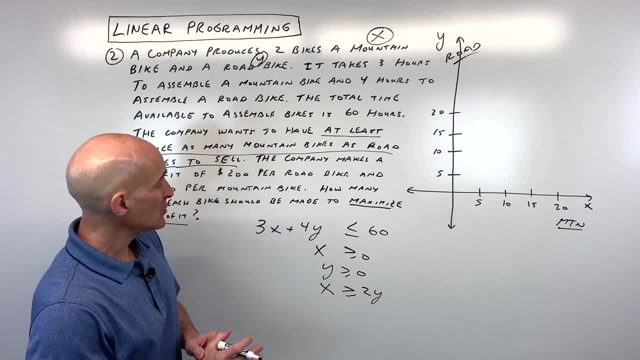 this to get Y by itself, But we'll do that in a minute. The first thing we want to do, though, is we want to look at a couple different ways to graph these, Like you see how this one's kind of like. 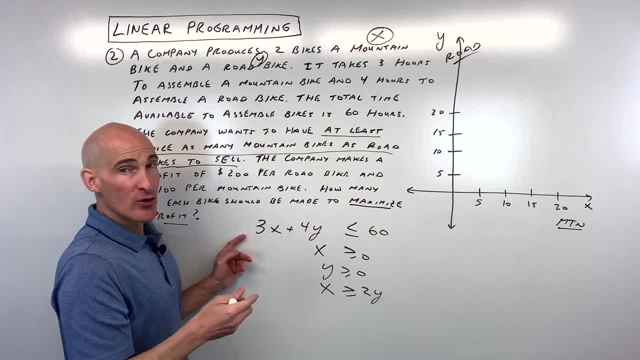 in the standard form. See how the variables are on the left, numbers on the right. Usually when it's in this form, I like to use the intercept method. I set X to zero and I solve for Y and I set Y to. 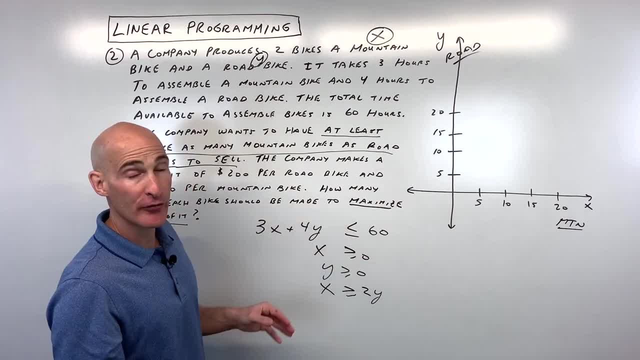 I set x to zero and I solve for y, And I set y to zero and I solve for x. You don't have to do that. If you want, you can rearrange the equation and solve for y And put it into: y equals mx plus b form. 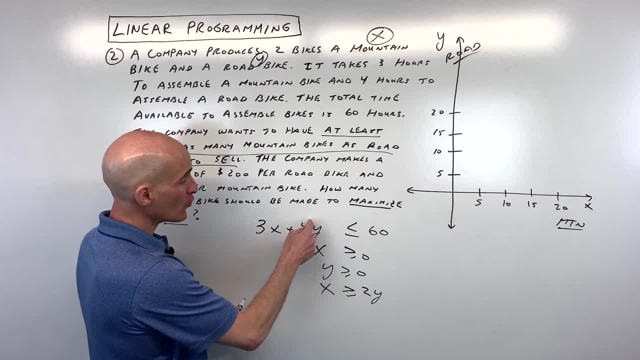 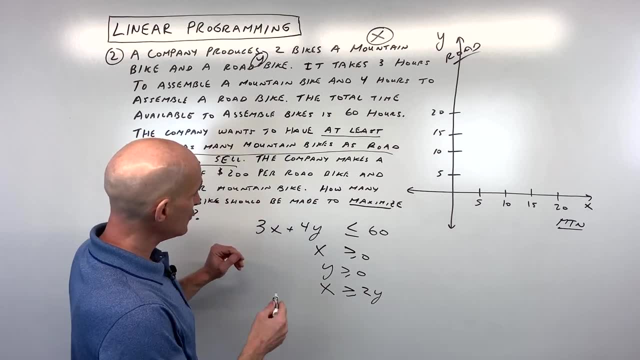 zero and I solve for X. You don't have to do that. If you want, you can rearrange the equation and solve for Y and put it into: Y equals MX plus B form. A lot of students prefer that method, But let's try and do the intercept method for this inequality. 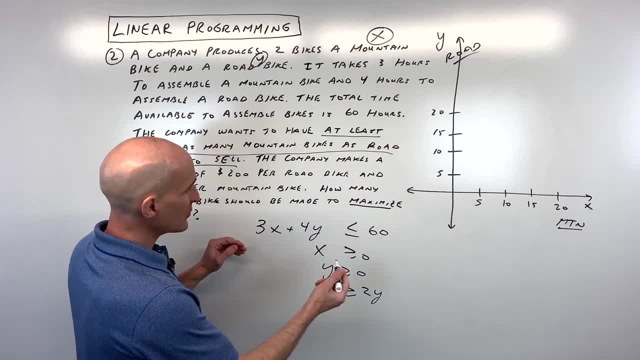 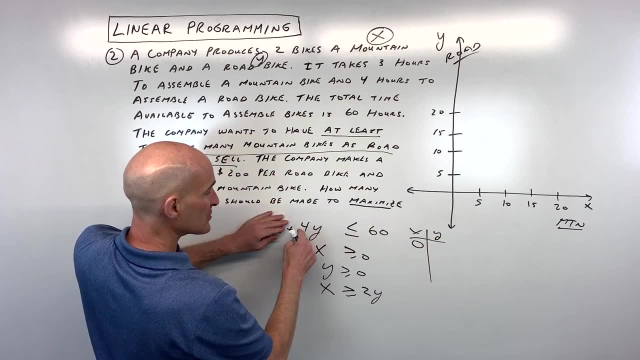 A lot of students prefer that method, But let's try and do the intercept method for this inequality. So x is zero. Three times zero is zero. I'm going to cover that up, Since it's nothing. Divide both sides by four. 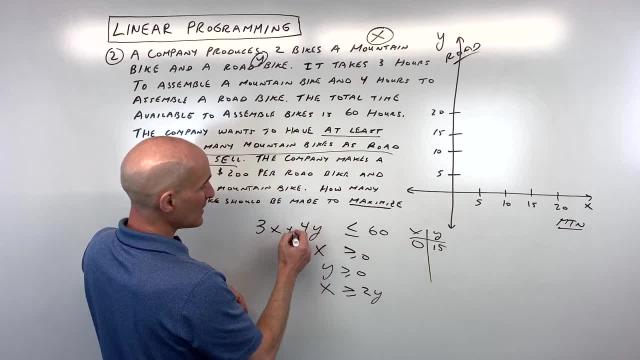 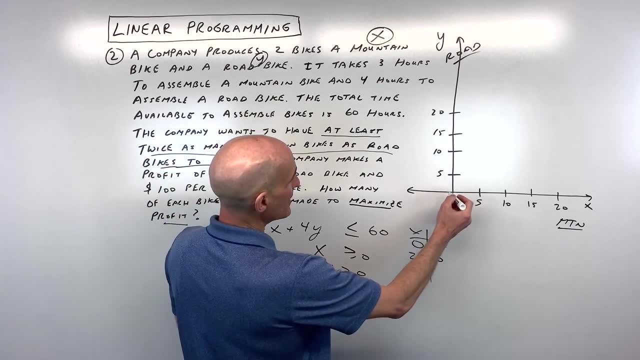 That means that y is 15.. If y is zero, four times zero is zero. That's nothing. Cover that up. Divide by three, You can see x is going to be 20 when y is zero. So let's plot those points. 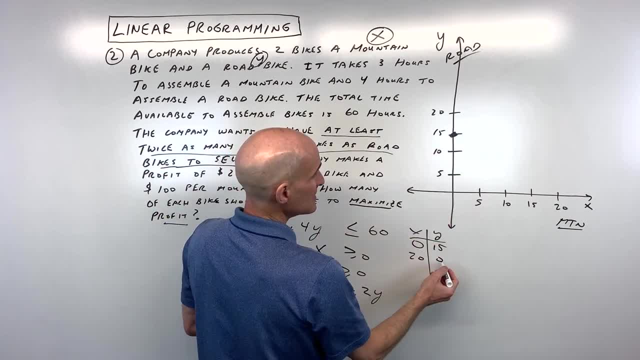 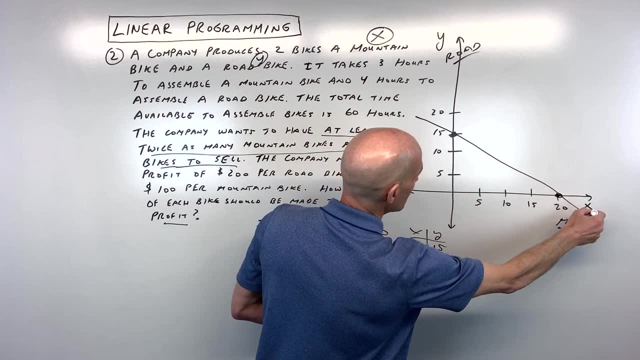 So zero, 15.. That's right there. 20, zero. That's going to be right there. We're going to draw a solid line, Since this is equal to right, And then what I'm going to do is I'm going to do a test point. 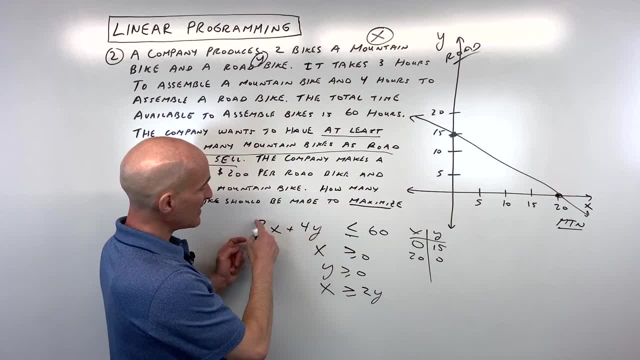 I'm going to pick the origin: zero, zero. If I put zero in for x and y, that makes this zero Is zero, less than or equal to 60?? Yes, So that means where this test point is. that's true. 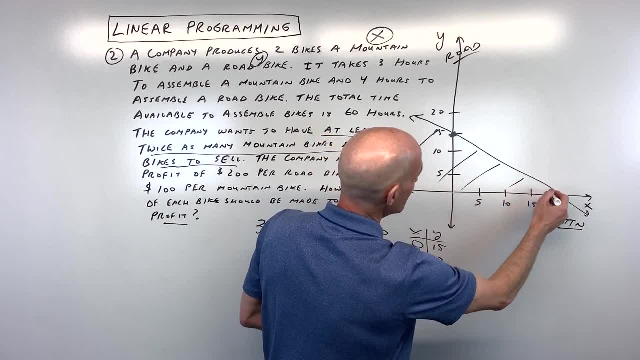 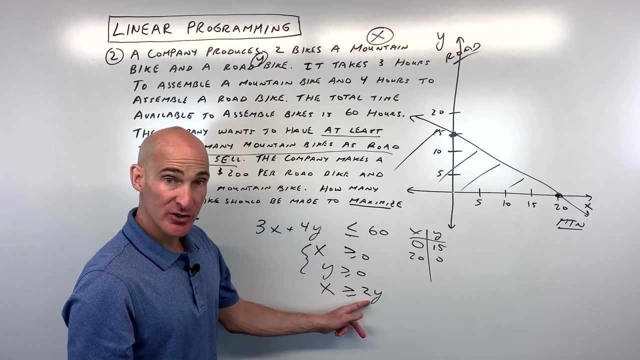 So you want to shade on that side of the line And remember we were in the first quadrant because of these two constraints. For the last one, though, you see how this is: x is greater than or equal to 2y. Let's get y by itself. 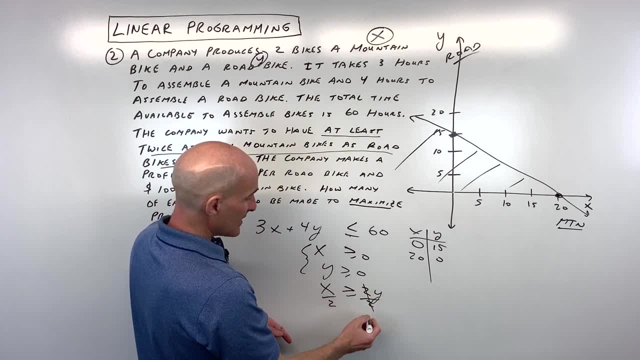 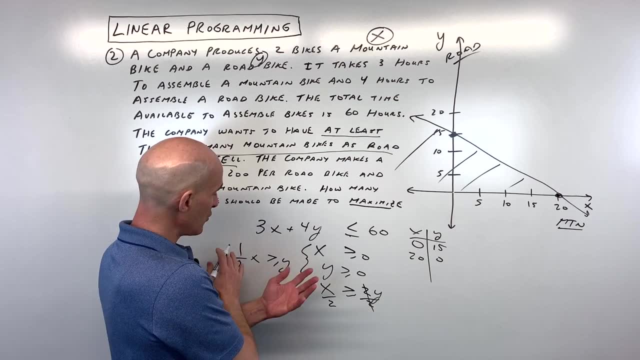 So we're going to divide both sides by two, And so that gives you one half x is greater than or equal to y. And then I'm going to flip this whole inequality So it's actually y. y is less than or equal to one half x. 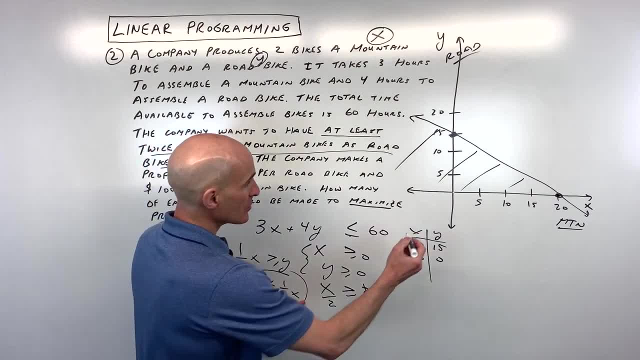 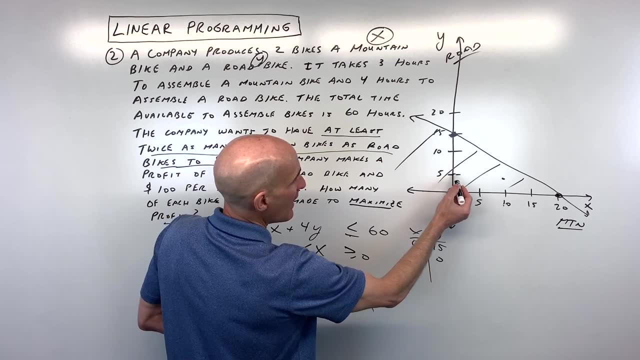 So let's go ahead and graph this one now. The y-intercept is zero, The slope is one half. So I'm going up one over two. Now see, really I went up five over ten, But because the scale on the x and y-axis is the same, 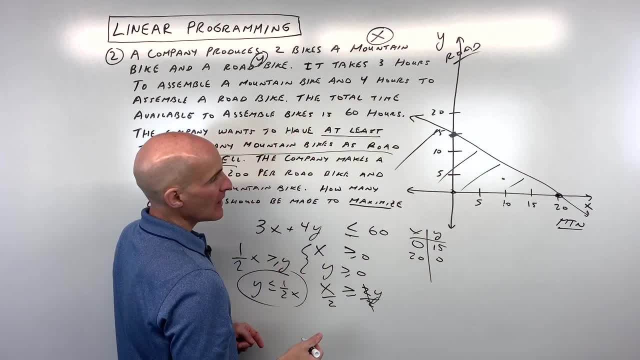 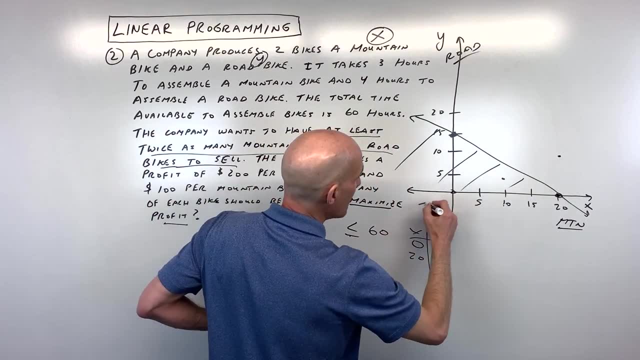 you can think of it as just going up one unit over two steps, And then let's repeat that: So up one over two. It puts you right about there, And this one is also equal to, so it's going to be a solid line. 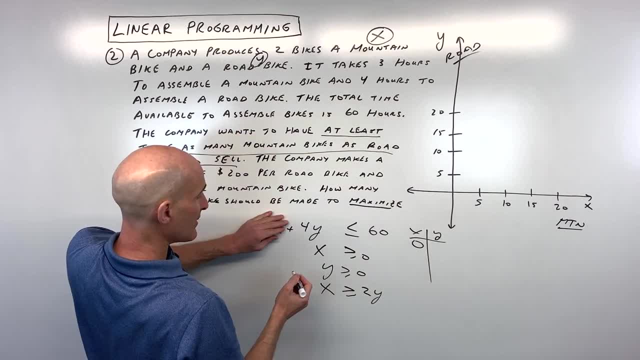 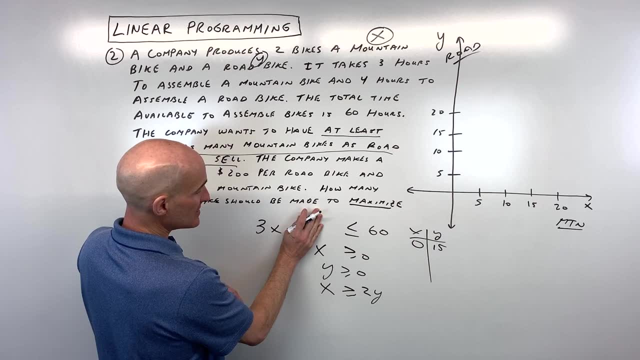 So X is zero. Three times zero is zero. I'm going to cover that up, since it's nothing. Divide both sides by four, That means that Y is 15.. If Y is zero, four times zero is zero, That's nothing. 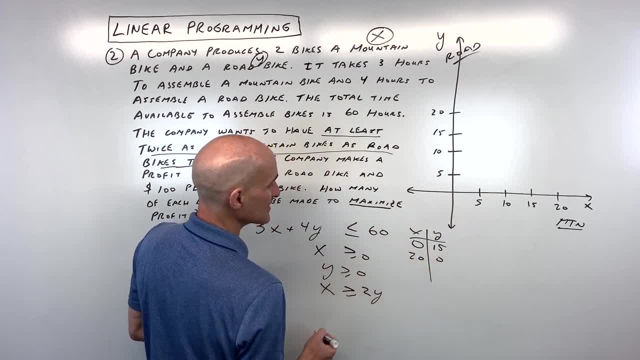 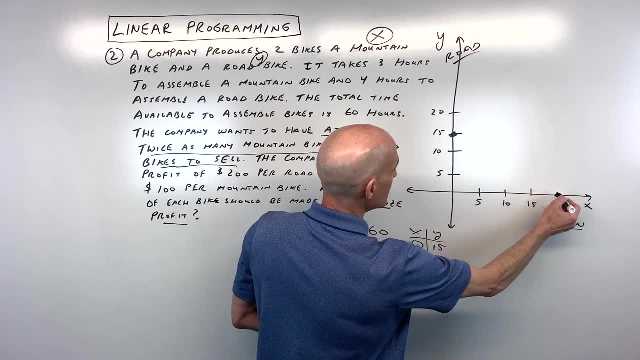 Cover that up, Divide by three. You can see X is going to be 20 when Y is zero. So let's plot those points. So zero, 15.. That's right there. 20, zero: That's going to be right there, We're going to. 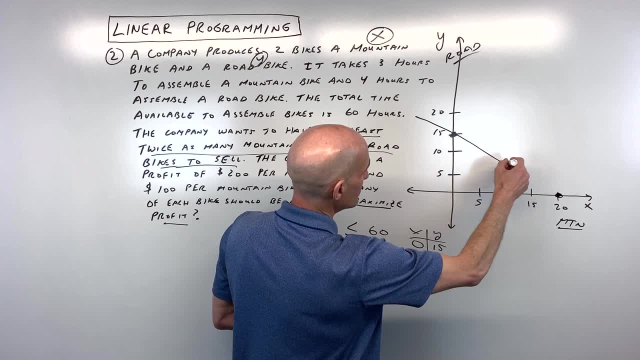 draw a solid line, since this is equal to right. And then what I'm going to do is: I'm going to do a test point, I'm going to pick a line and I'm going to do a test point. I'm going to pick a. 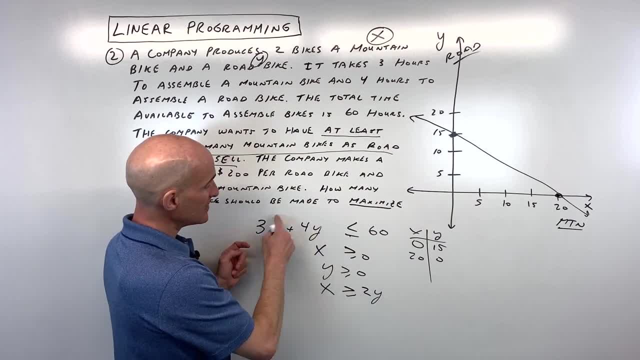 origin: zero, zero. If I put zero in for X and Y, that makes a zero. Is zero less than or equal to 60?? Yes, So that means where this test point is, that's true. So you want to shade on that side of? 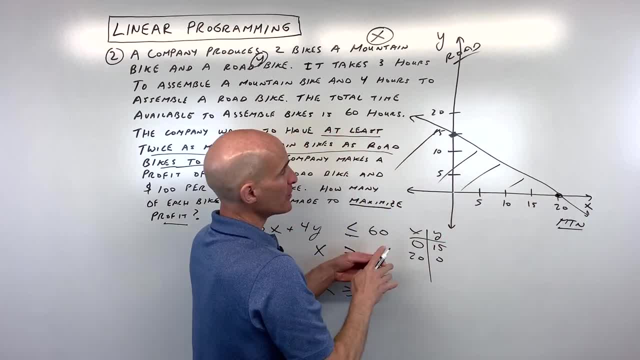 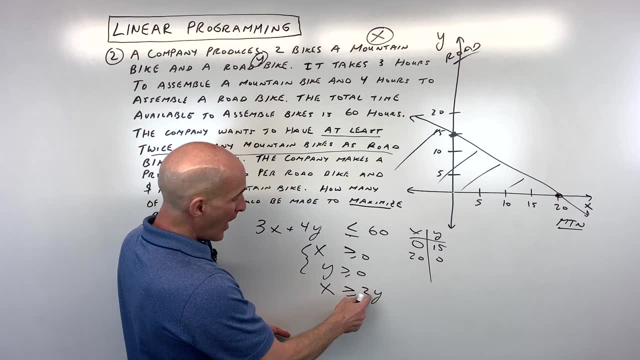 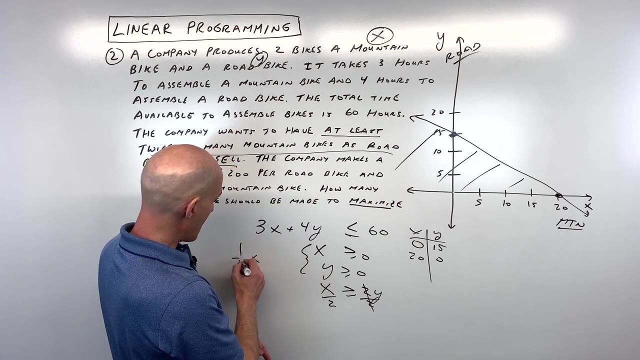 the line, And remember we were in the first quadrant because of these two constraints. For the last one, though, you see how this is: X is greater than or equal to 2Y. Let's get Y by itself, So we're going to divide both sides by two, And so that gives you one half. X is greater. 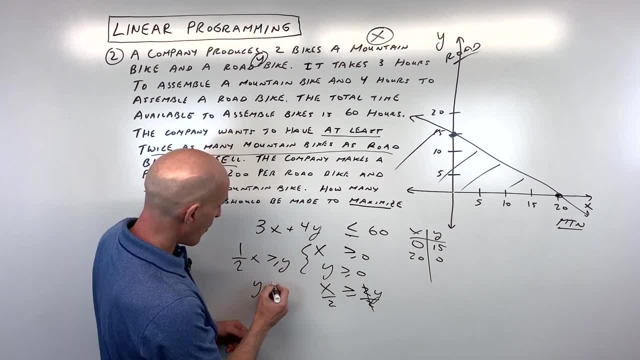 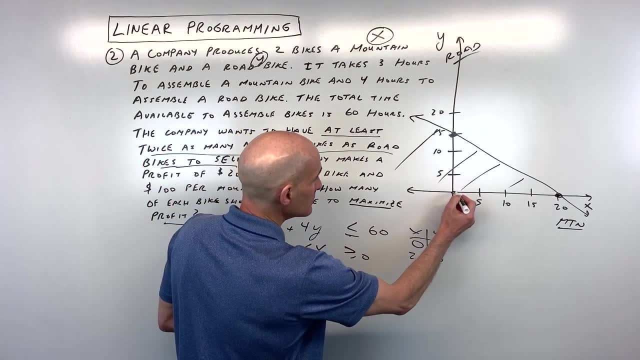 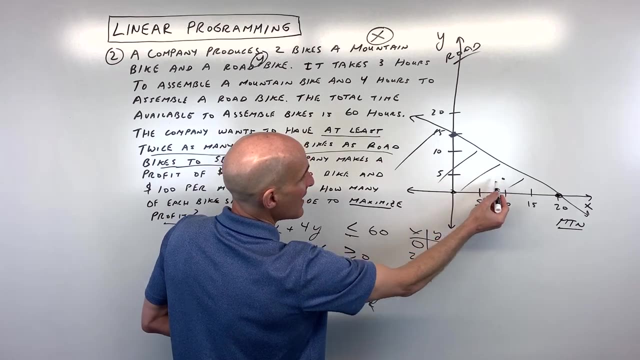 than or equal to Y. And then I'm going to flip this whole inequality. so it's actually: Y is less than or equal to one half X. So let's go ahead and graph this one now. The Y intercept is zero, The slope is one half. So I'm going up one over two. Now see, really I went up five over 10.. 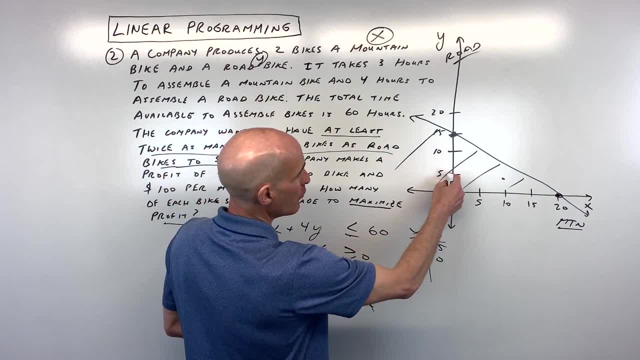 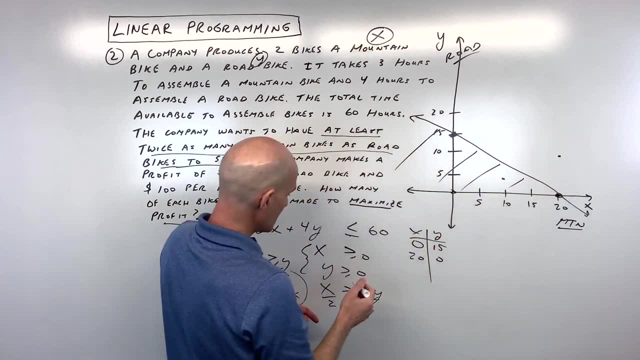 But because the scale on the X and Y axis is the same, you can think of it as just going up one unit over two steps, And then let's repeat that. So up one over two. It puts you right about there. And this one is also equal to, so it's going to be equal to two. So I'm going to put this one up one over two. 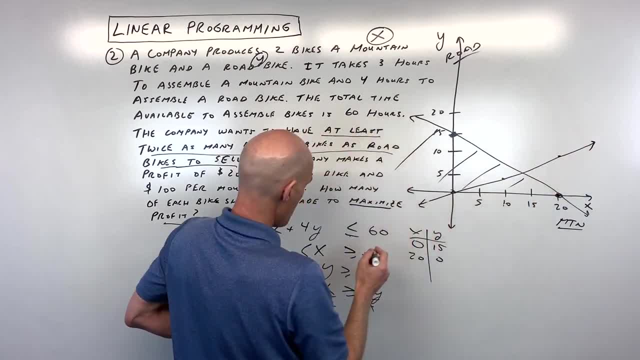 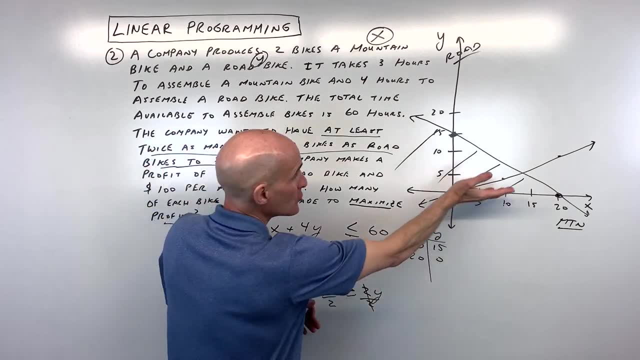 So it's going to be a solid line like this: right, But Y is less than Now. when you have the Y by itself, OK, on one side of the inequality, if Y is less than Y controls up and down right, So less. 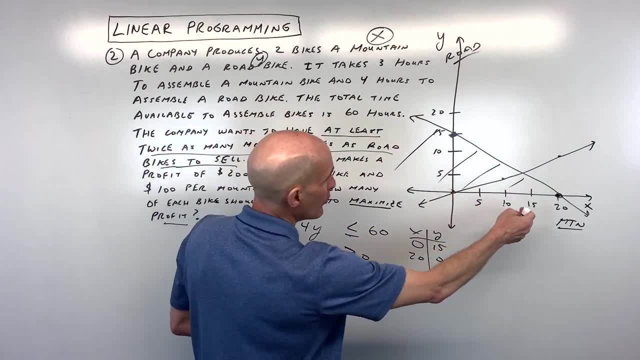 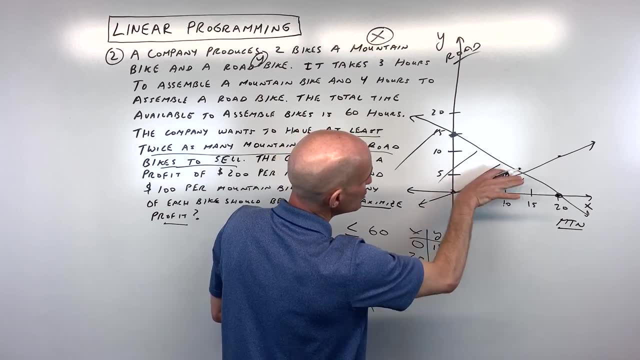 than means we're shading below this line. If you want, you can do a test point. You can pick a point over here, see if it makes the inequality true. If it's false, you shade the other side. If it's true, you would shade where that test point is. So that means we're going to be shading below this. 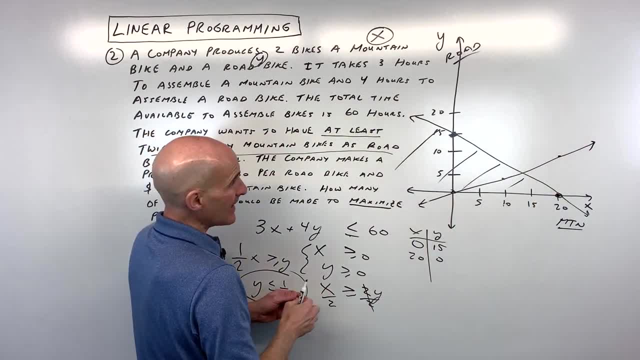 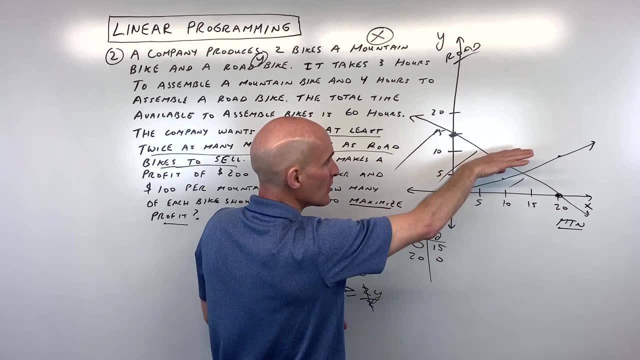 Like this right, But y is less than Now when you have the y by itself. okay, on one side of the inequality, if y is less than y controls the up and down right. So less than means we're shading below this line. 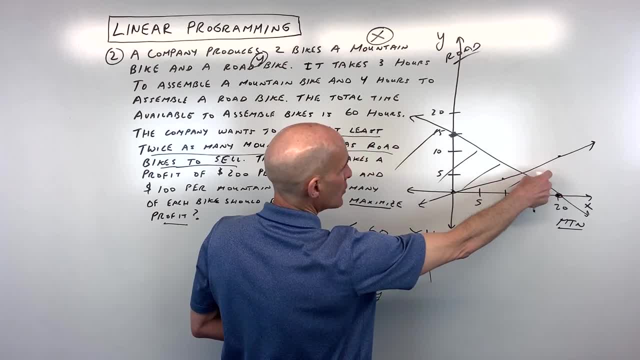 If you want, you can do a test point. You can pick a point over here. see if it makes inequality true. If it's false, you shade the other side. If it's true, you would shade where that test point is. 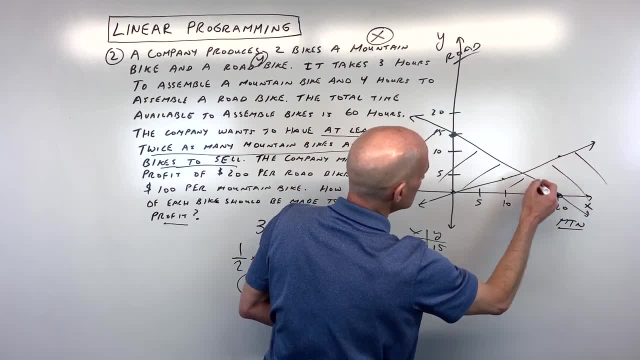 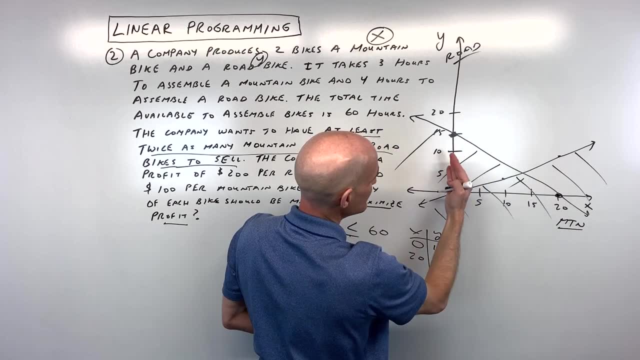 So that means we're going to be shading below this line right Now. you can see where are they overlapping. We're below this line. We're below this line. We're above the x-axis. We're to the right of the y-axis. 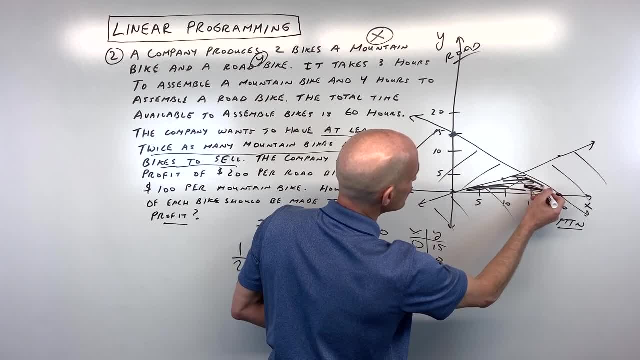 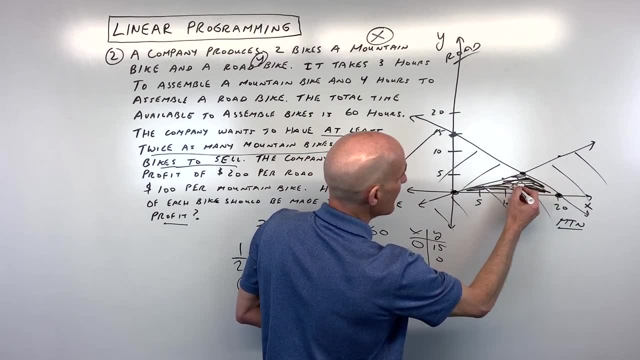 It's going to be right. in this region, right here, It kind of forms like a triangular region. The main thing that we're interested in now are the vertices of that feasible region. okay, that polygon that's formed right. So we know this point. 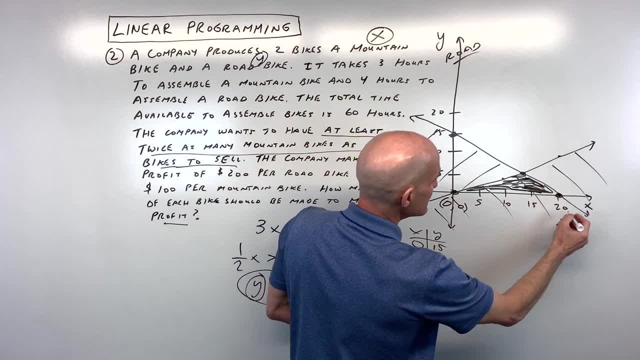 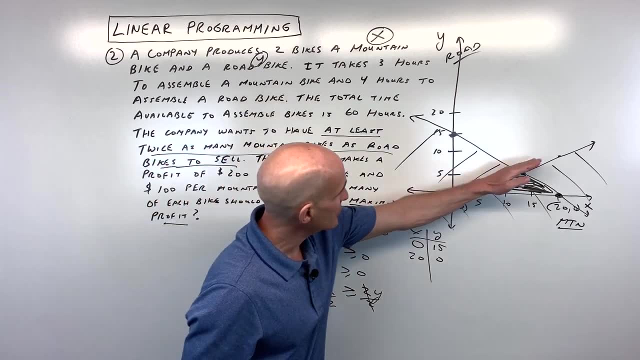 That's easy: Zero, zero. We know this point. That's easy. That's 20 comma zero. How do we find this point? That's probably the toughest part about the problem, right? Well, it looks like this is the intersection of these two lines. 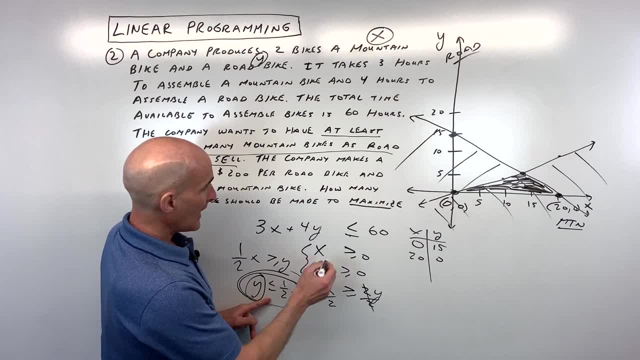 y equals one half x. We're just going to do that. We're just going to treat it like an equation, And this one here: 3x plus 4y equals 60. I think the easiest thing to do is to do a substitution. 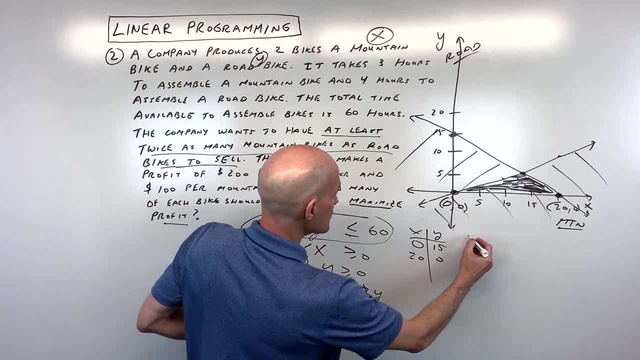 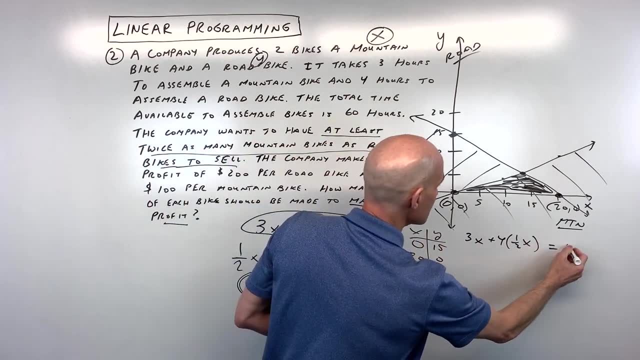 So if y equals one half x, I'm going to put one half x here. So that comes out to 3x plus 4 times one half x, because we're putting one half x in for y equals 60. We're just treating it like an equation. 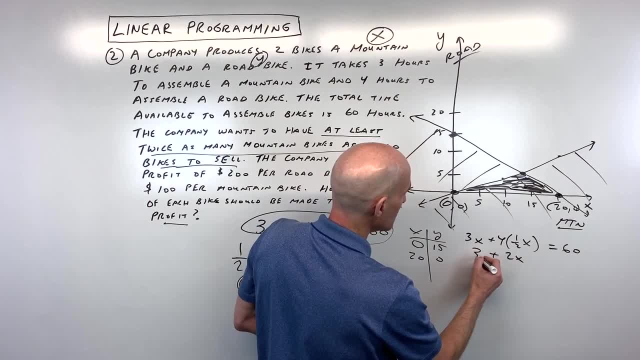 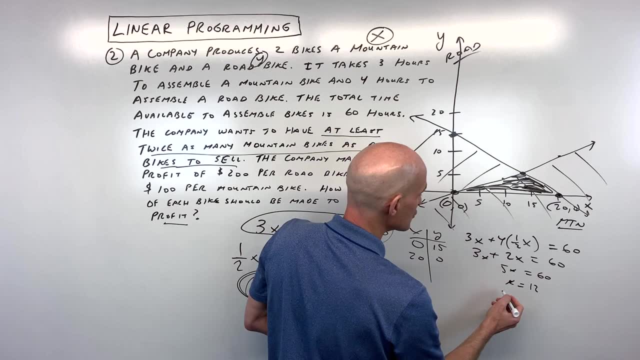 Four times one half is 2x plus 3x, That's 5x divided by 5. You can see x is coming out to 20.. If we put 12 back in- here or here, it doesn't matter Either. one one half times 12 is 6.. 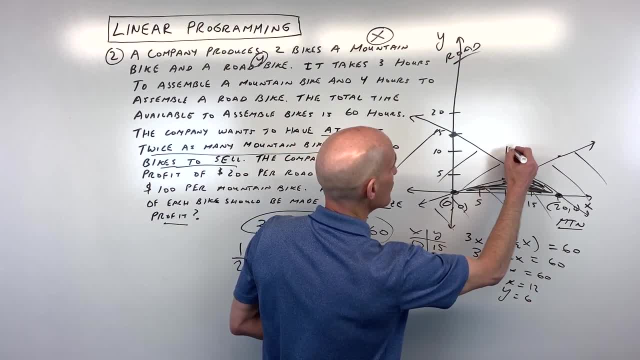 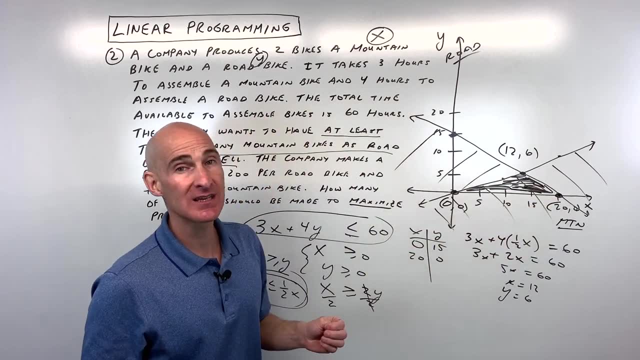 So our y value equals 6.. So this point is really right here at 12 comma 6.. Now all we have to do is test which one of these points is going to give us the maximum profit, because that's what we're trying to maximize. 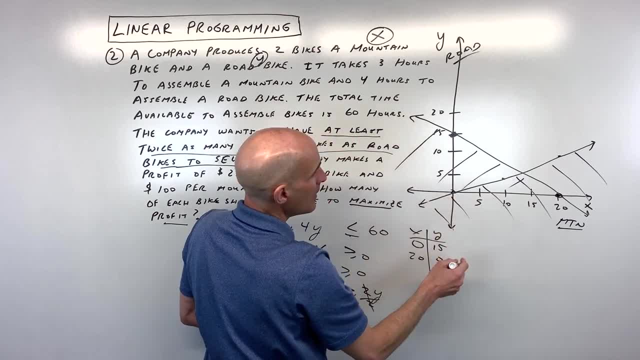 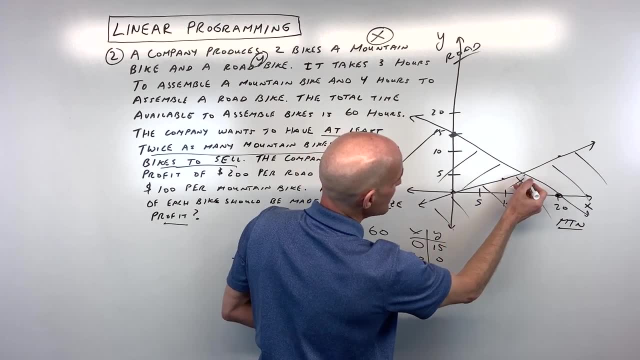 line. right Now you can see where are they overlapping. We're below this line. We're below this line. We're above the X axis. We're to the right of the Y axis. It's going to be right in this region, right here, It kind of forms like a triangular. 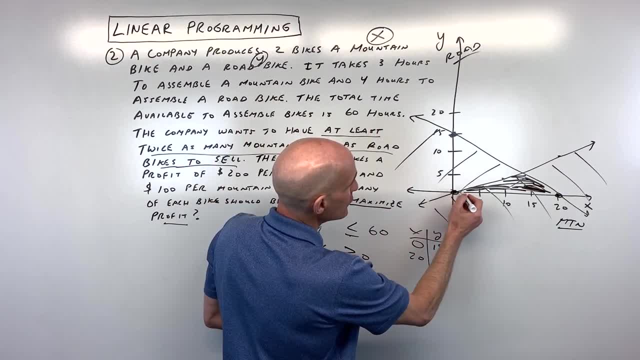 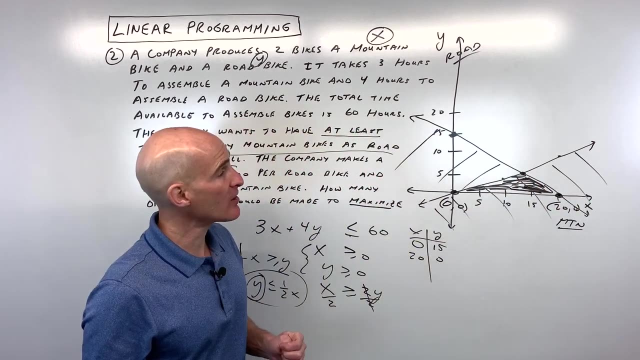 region. The main thing that we're interested in now are the vertices of that feasible region. OK, that polygon, that's formed right. So we know this point, That's easy: 0, 0.. We know this point, That's easy. That's 20, 0.. But how do we find this point? That's probably the toughest part. 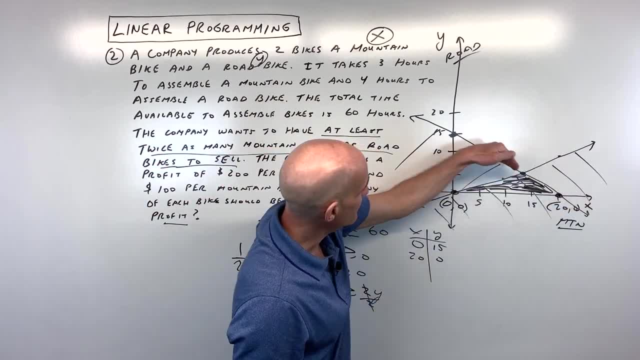 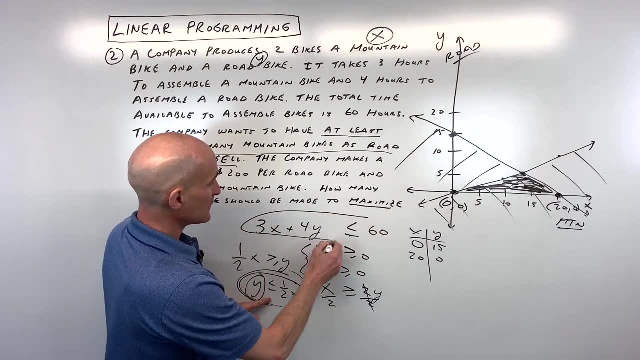 about the problem, right? Well, it looks like this is the intersection of these two points. These two lines: Y equals 1 half X- We're just going to treat it like an equation- And this one here, 3X plus 4Y, equals 60. I think the easiest thing to do is to do a substitution. So if Y 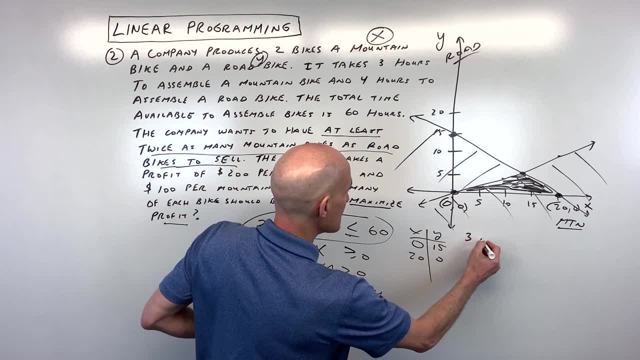 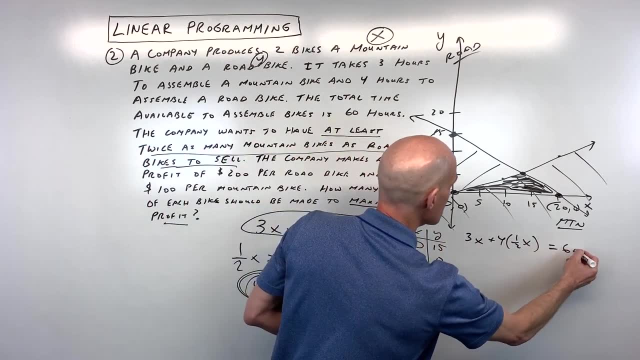 equals 1 half X. I'm going to put 1 half X here, So that comes out to 3X plus 4 times 1 half X. because we're putting 1 half X in for Y equals 60. We're just treating it like an equation. 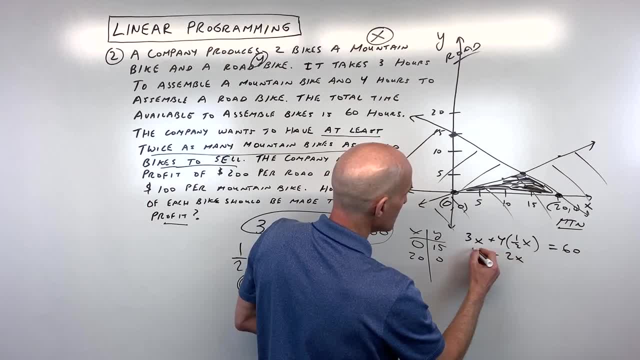 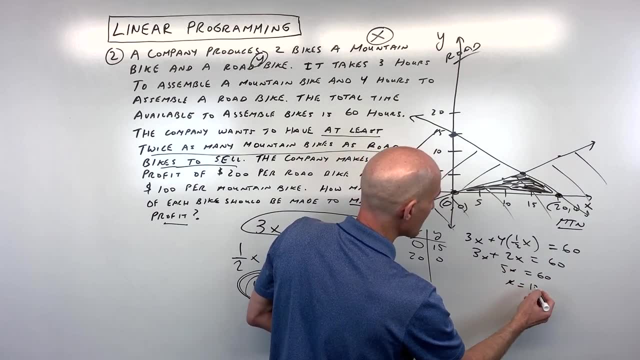 4 times 1 half is 2X plus 3X. That's 5X Divide by 5.. You can see X is coming out to 12.. If we put 12 back in here or here, it doesn't matter. 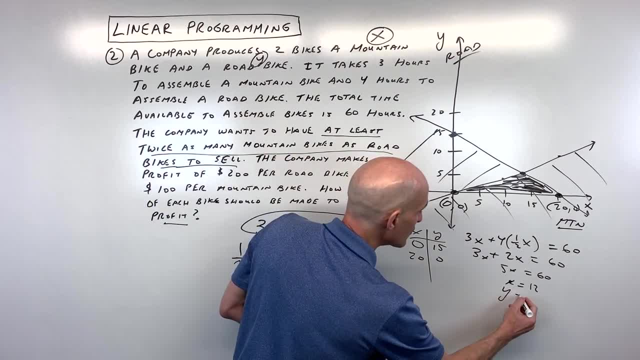 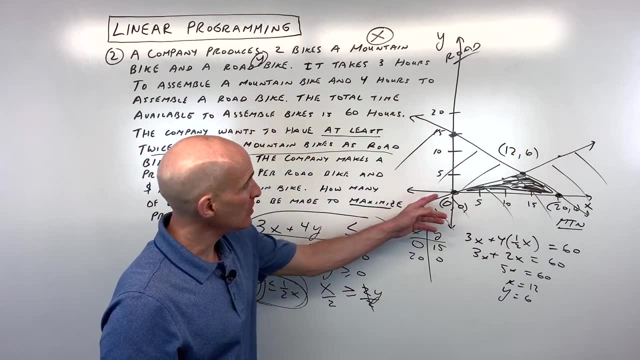 either one 1 half times 12 is 6.. So our Y value equals 6.. So this point is really right here at 12 comma 6.. Now all we have to do is test which one of these points is going to give us the maximum. 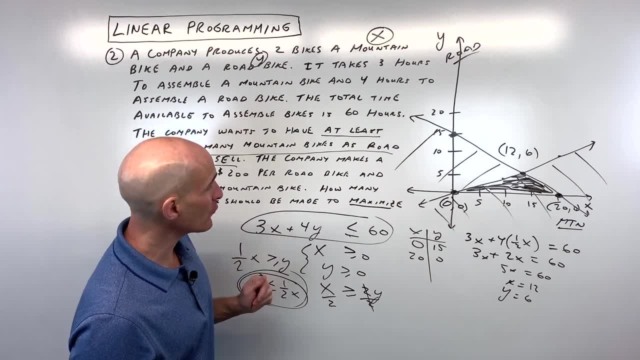 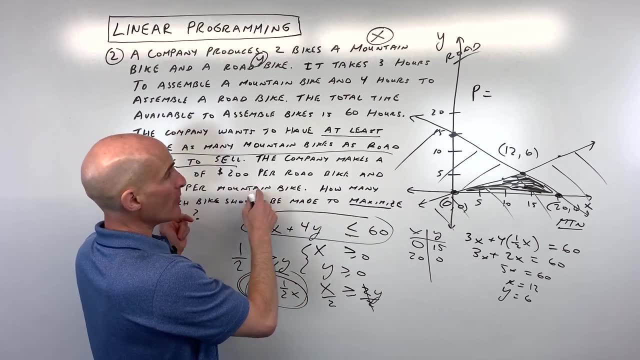 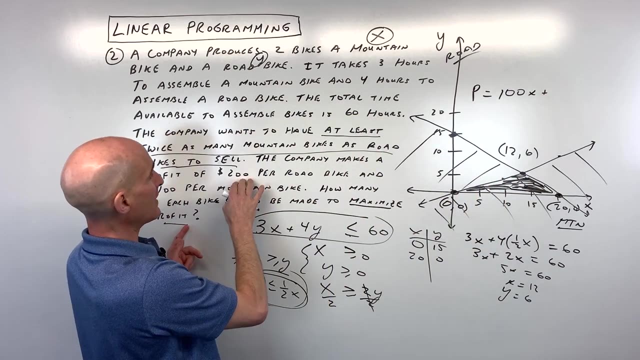 profit, because that's what we're trying to maximize. Now we didn't write the formula for the profit equation yet, So let's do that. Profit equals: you make $100 per mountain bike, So that's 100 times X, And you make $200 for each road bike. 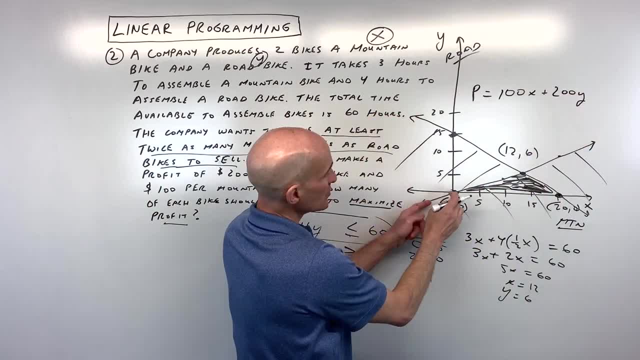 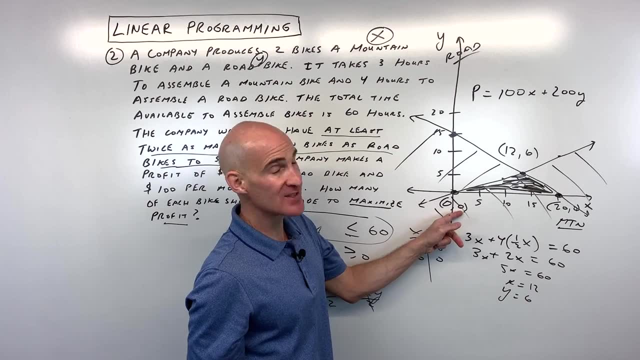 So that's going to be plus 200Y. So what we're going to do is we're going to take each points on the vertices of this feasible region and we're going to plug it into our profit equation. Of course, if you sell zero mountain bikes and zero road bikes, 100 times 0,, 200 times 0, that's a 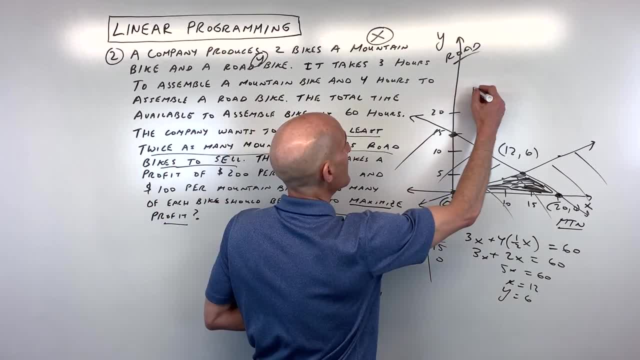 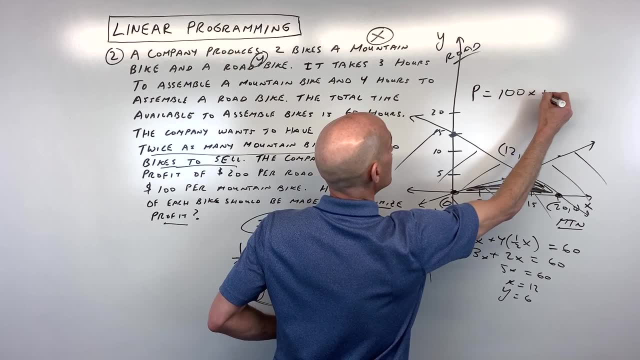 Now, we didn't write the formula for the profit equation yet, So let's do that. Profit equals: you make $100 per mountain bike, So that's 100 times x, And you make $200 for each road bike, So that's going to be plus 200 y. 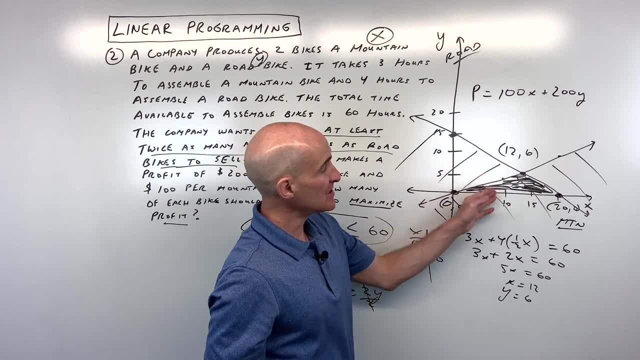 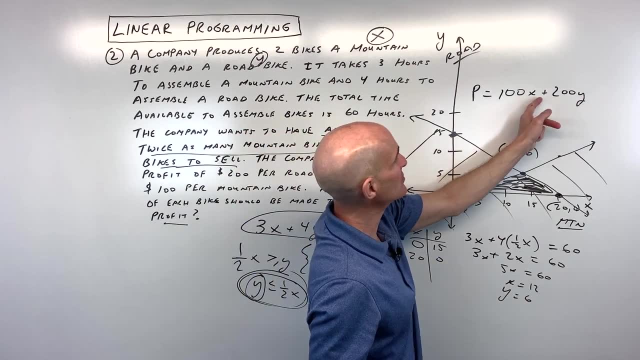 So what we're going to do is we're going to take each points on the vertices of this feasible region and we're going to plug it into our profit equation. Of course, if you sell zero mountain bikes and zero road bikes, 100 times zero, 200 times zero, that's a profit of zero. 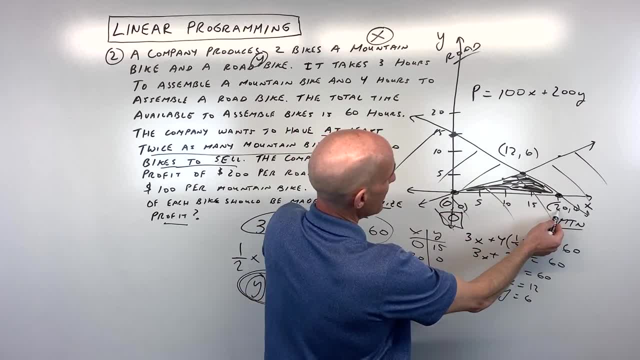 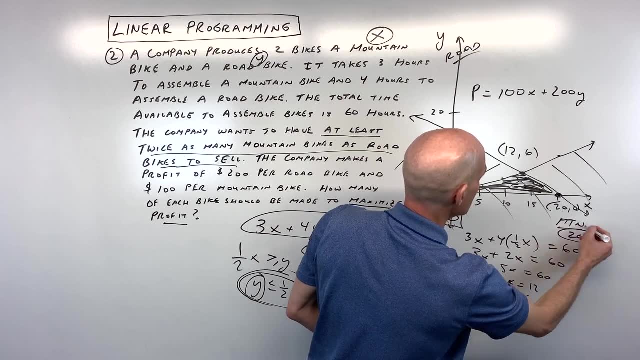 If we do this point over here, 20 mountain bikes and zero road bikes, that's going to be 20 times 100 is 2,000 plus zero. So this is going to give us A profit of 2,000..